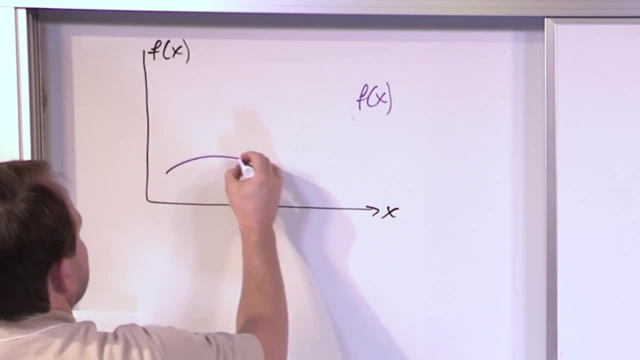 Let me go ahead and draw this guy just a little bit closer to the axis, like this. What this is going to yield is basically a mirror image, something like this, And so you get a shape that would kind of look like a vase, let's say. for a shape like this, Of course, f of. 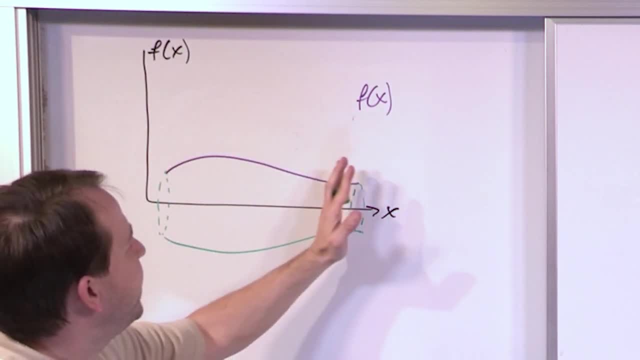 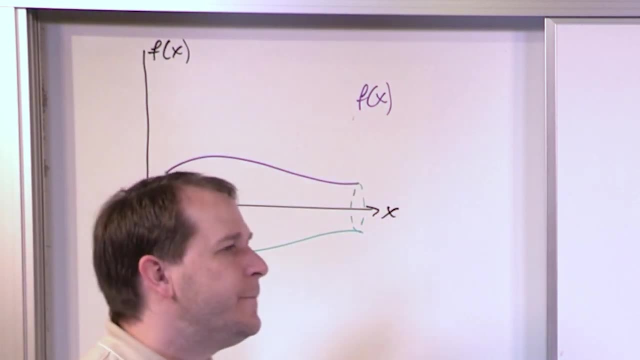 x could be any shape you want. We already know we can use the disk method to calculate the volume of this object by integrating from a to b. But what we want to know is how to calculate that surface area. In other words, if I had to buy paint to paint the outside. 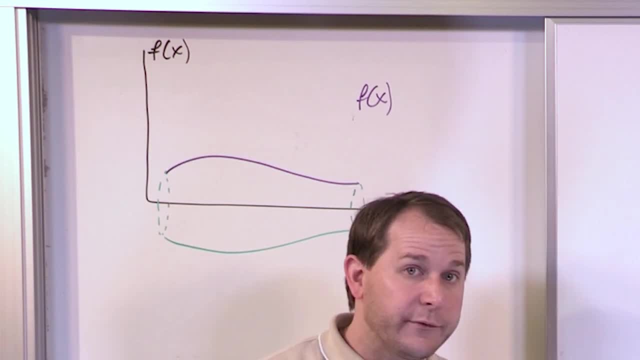 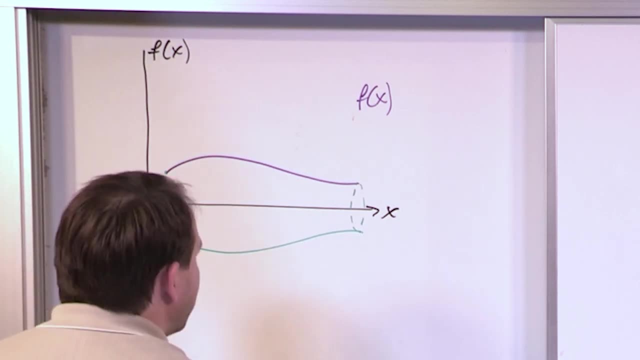 of the object. how many square centimeters of paint coverage would I need that to have? That's what surface area, is right? So let me just write down you know what the answer is. The answer to this guy is: what we're going to do is let f of x be non-negative, which. 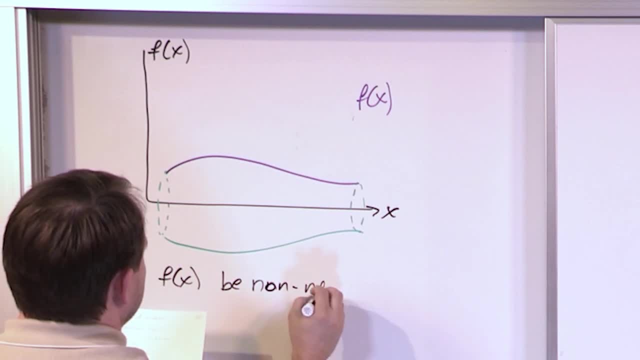 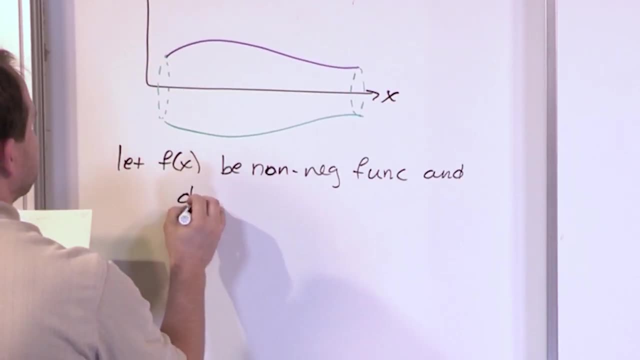 means a positive function above the x axis, a non-negative function, and differentiable means we can take derivatives of it on some interval: a- b. The reason we have a- b here is because this first part of the curve we're calling a and 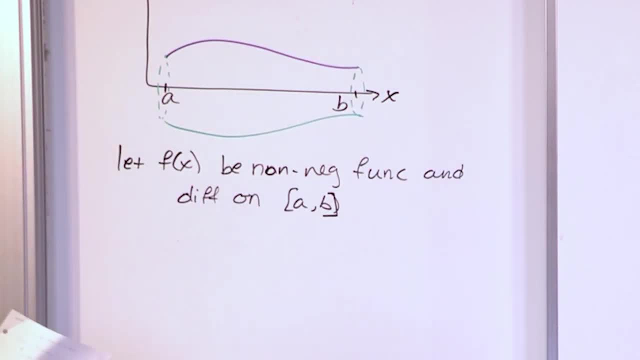 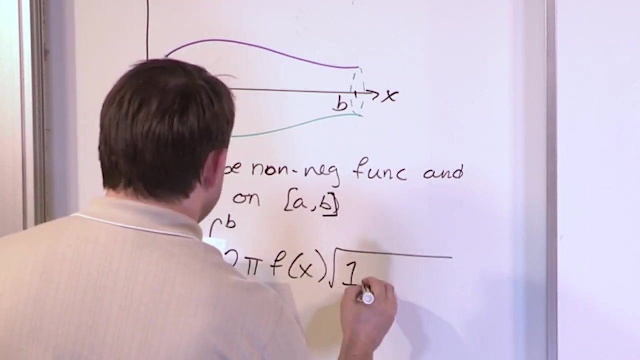 we're going to end up integrating to b. This is the same thing that we're always doing. Then the surface area- sa I'm going to call the surface area- is going to be the integral, you might guess, from a to b, of 2 times pi, times f, of x, times the square root of 1 plus. 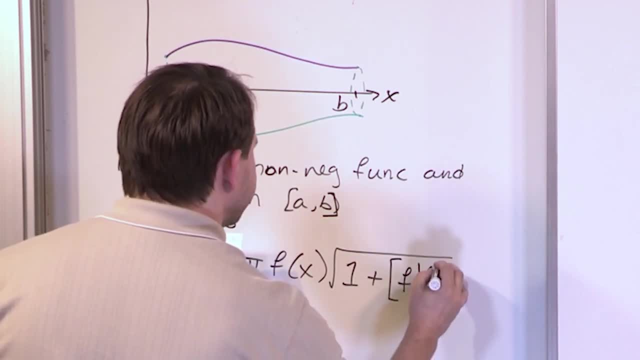 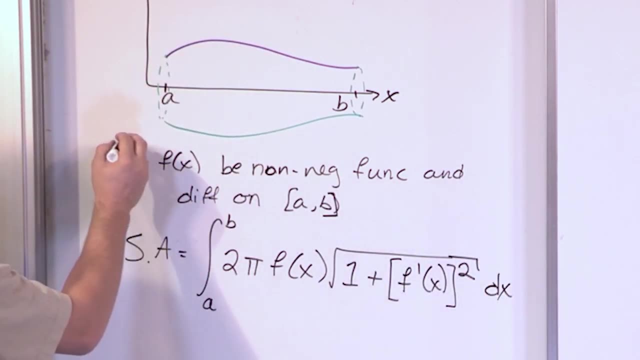 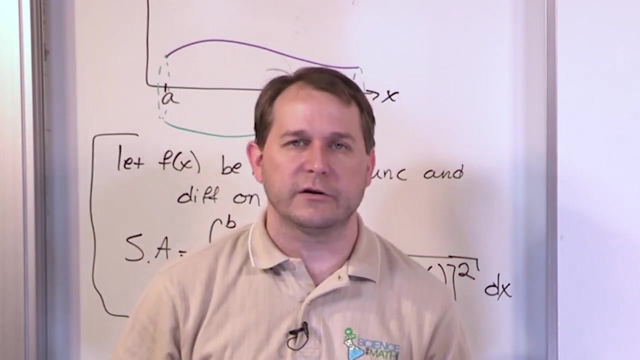 now watch carefully what's inside of here. f, prime of x, close the bracket, square it. all this is under the square root dx. Now, if you notice, when we talked about the disk method and we talked about the washer method, and even when we talked about the shell method, I went through great lengths. 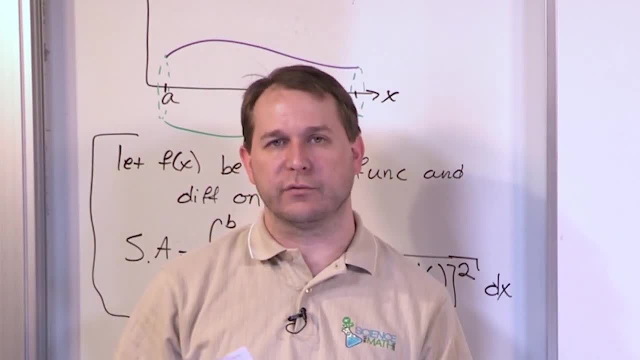 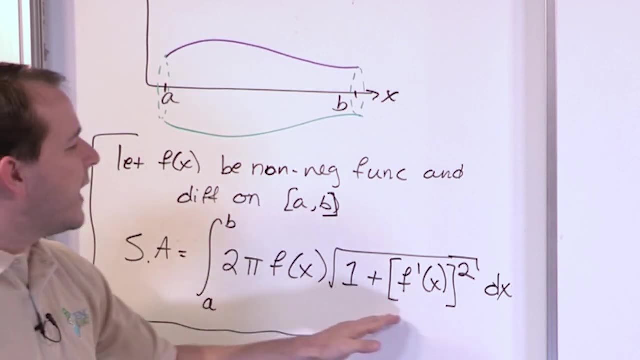 drawing a picture and showing you how those relations, how those integrals, actually do calculate the volume of your object, and we were doing that before. You can do a similar thing to derive this kind of integral, but what ends up happening is, it's not quite as obvious. 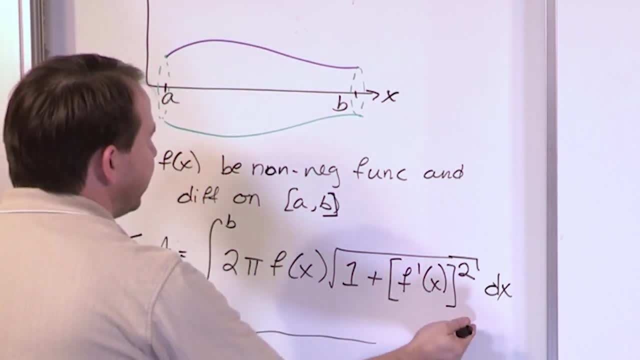 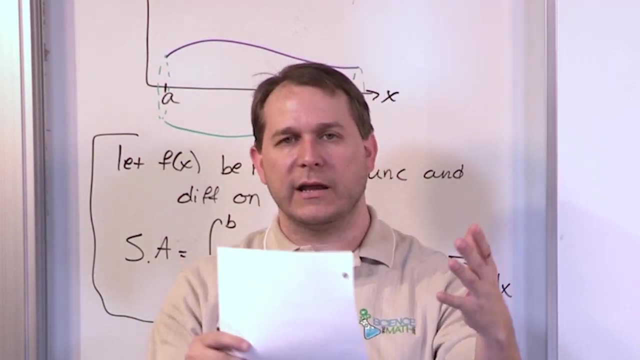 to draw a quick picture and show you how this happens. so if I were going to prove this to you, I'd have to break it out and I'd have to divide the drawing up into these little quadrants and I'd have to make a lot of assumptions and draw a lot of intermediate equations. 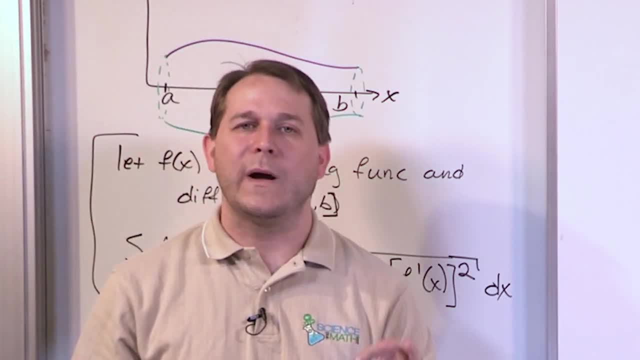 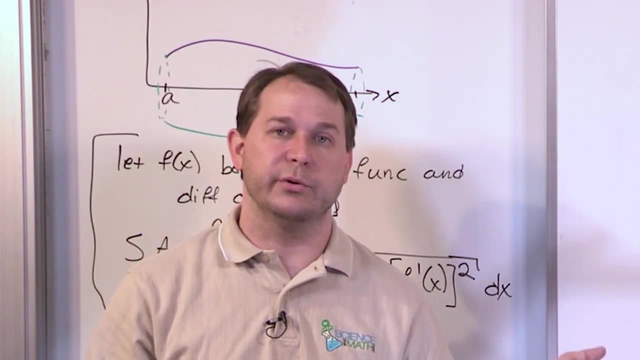 and eventually it would condense down into this and it's not quite as straightforward as it is for shell method and disk method and washer method, so those are kind of easier to understand, basically what we were doing before. It's not hard or impossible for you. 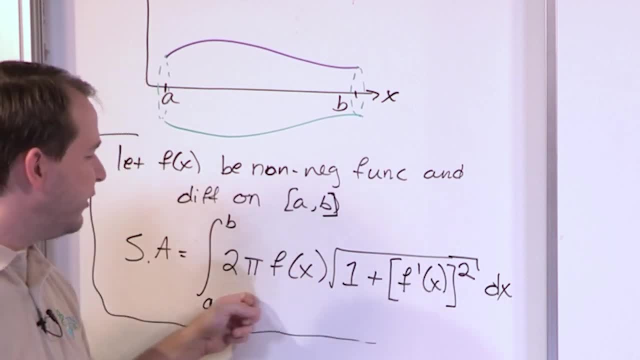 to understand where this comes from, but I have to make judgment calls sometimes, and my judgment call this time is: I'm going to draw a quick picture and show you how this works. So what I'm going to do this time is that it's going to be too much of a detour for. 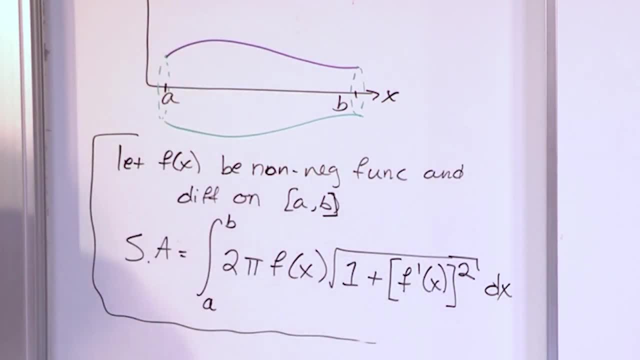 not very much of a gain to be able to derive this for you. So this is going to be one where I'm just going to present it to you and say: this is the surface area of an object in three-dimensional space that's revolving a function around the x-axis and we're integrating 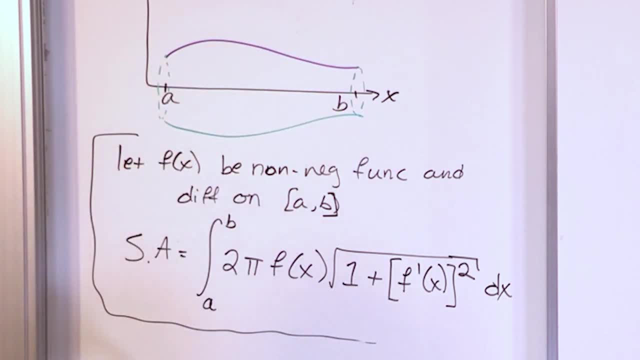 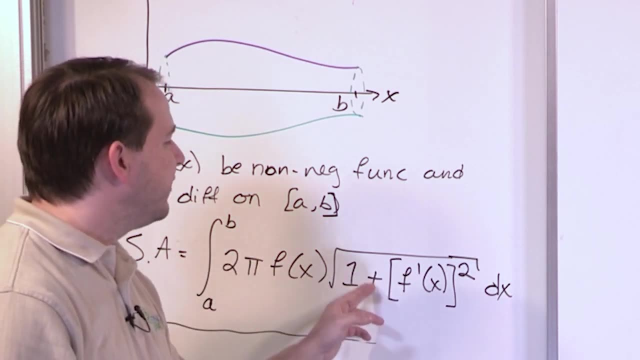 along the x-axis from a to b, which is the extent of the object, 2 times pi, times the function that we're defining, the boundary to be or the shape to be, times the square root of 1 plus f, prime of x. 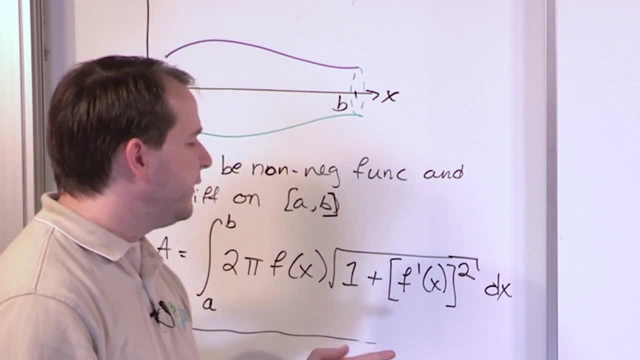 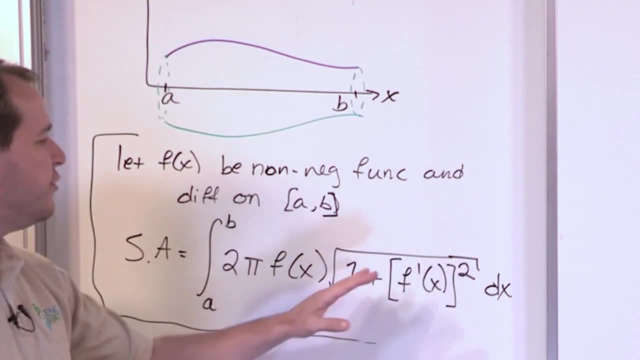 So this is the first derivative of the function. So really the way you do this is you take your function, you take the derivative, then you square it, then you add 1 to it, then you take the square root of the whole thing and you're multiplying that whole quantity. 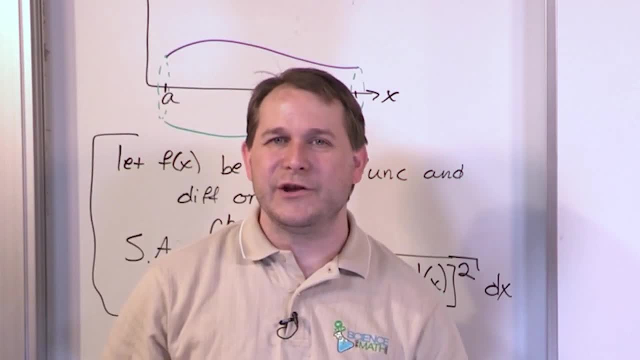 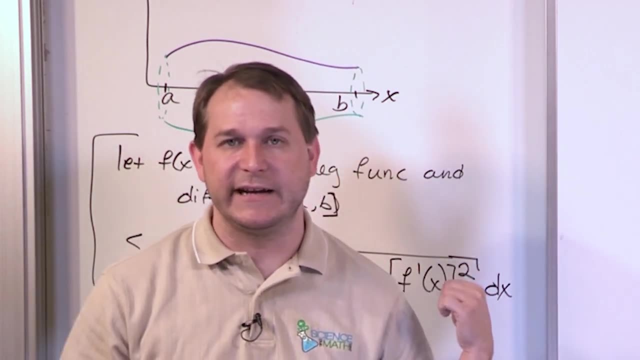 times 2 times pi, times the function itself, And then you do all that and you integrate it. So, as you can see, you know it can be a little tricky And if you just take any function you want, any f of x and stick it in here, you're going to get very complicated. 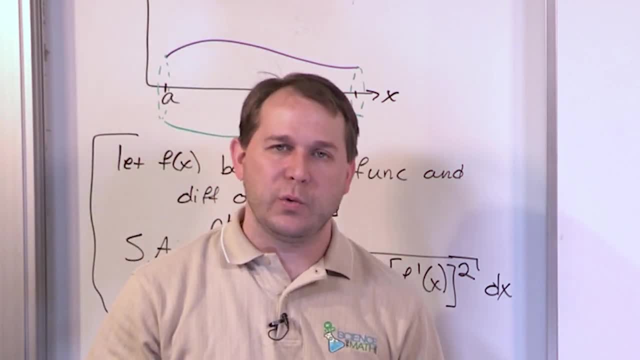 integrals. So when you're calculating surface area on an exam or on a quiz, the problems are going to be chosen. So you're going to have to do a little bit of math and you're going to have to figure it out without the simple mistake of using the same advantage. 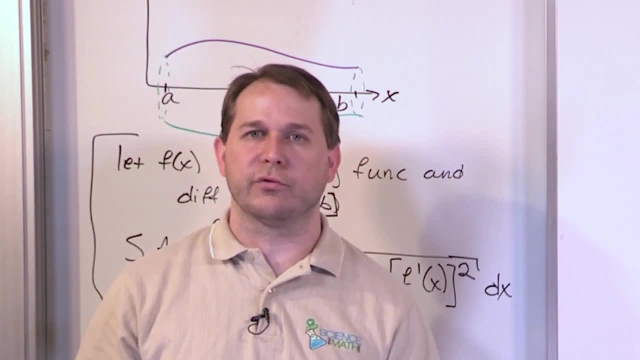 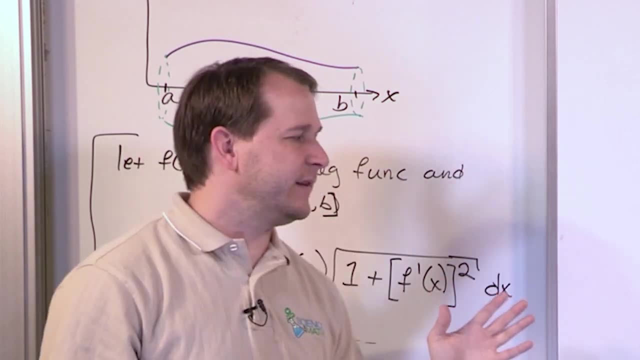 as we did before. So let's try this: If you put a bad integral in here- because you know you always have to do a simple mistake here- if you put anything in here that's the same as you did before, you're probably going to get a crazy integral that has no relation, no resemblance to anything. 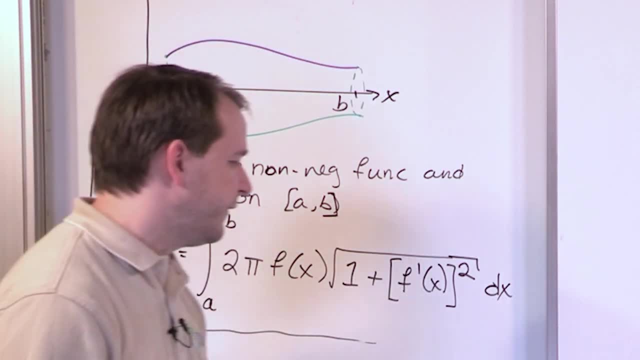 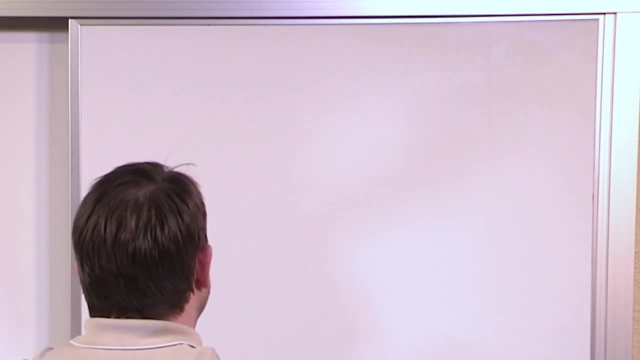 that you've done before. You've probably made a simple mistake because, like I said, if I just take any old function and stick it in here, you're going to get very complicated integrals that you don't know how to solve. So you're kind of looking for that simplification. 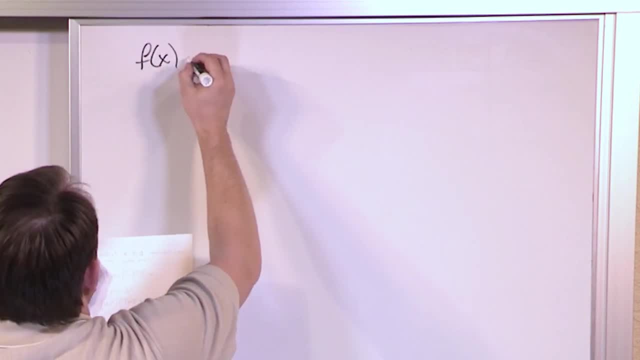 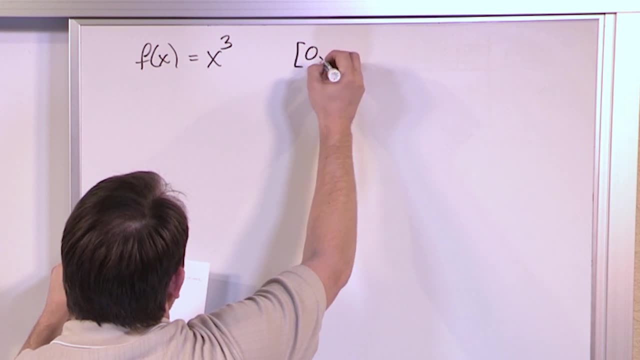 to happen on its own. f of x is our function, x cubed- very nice function. everyone knows what that looks like. The boundary that we care about the extent of the object is from x is equal to zero to x is equal to one. 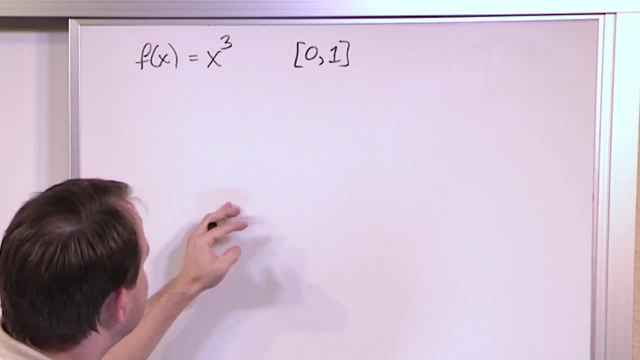 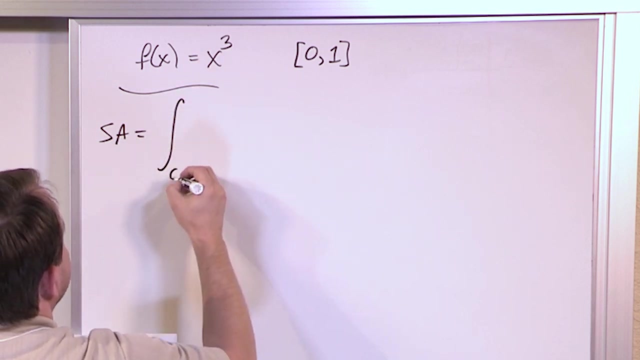 So if you can imagine what x cubed looks like, from zero to one, that little sliver, and then we're revolving that sliver around the x axis and we want to find the surface area of the resulting three-dimensional object. So what we're going to have, the surface area is going to be equal to the integral from. 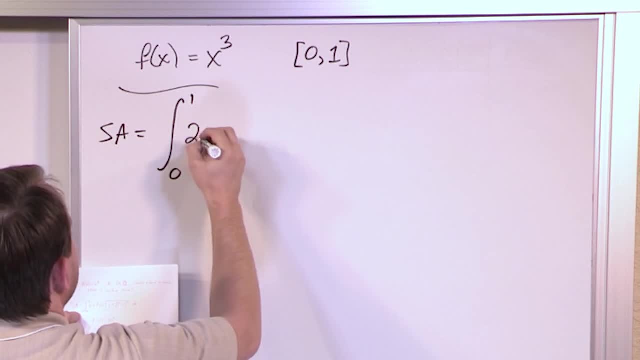 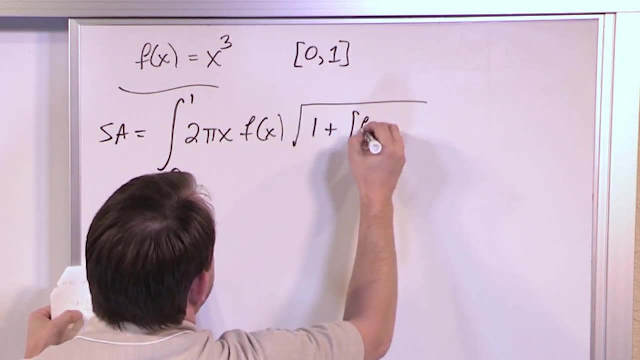 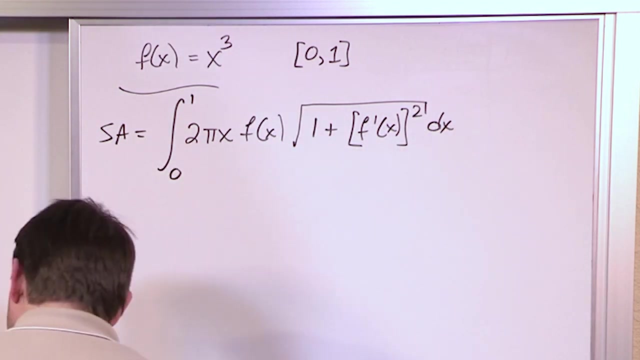 zero to one, which is our limit here, and we'll have two pi x, f of x times the square root of one, plus open a bracket, f, prime of x square that quantity dx. So it's a few things to do. 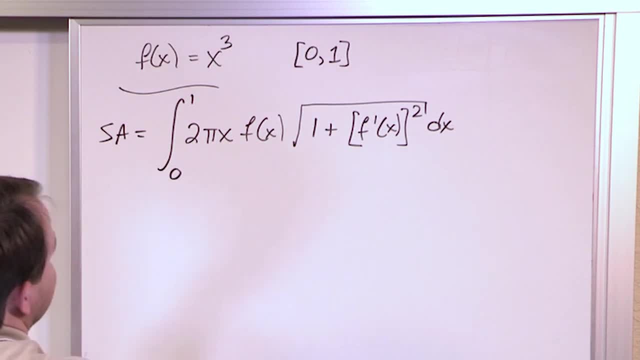 But you know what? None of it's hard. That's the good news. So let's go ahead and take this guy. If this is f of x, then f prime of x is going to be derivative of this is three x squared. 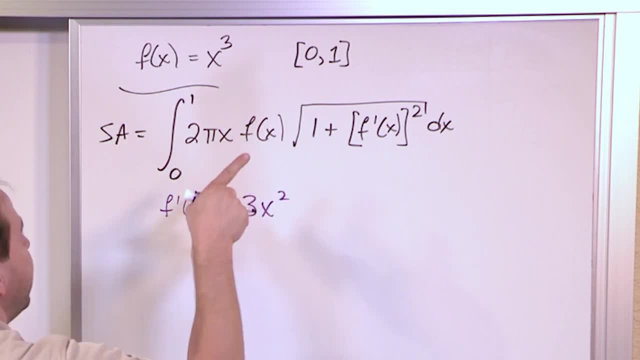 squared. That's what the derivative is, And so when we plug everything in here, what we're going to get is the surface area is going to be the integral from zero to one of two pi x times f of x, which was x cubed. 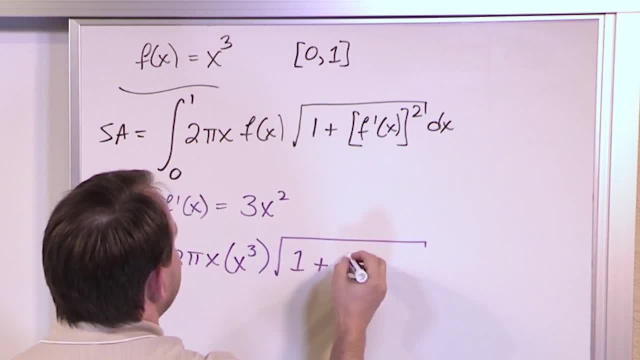 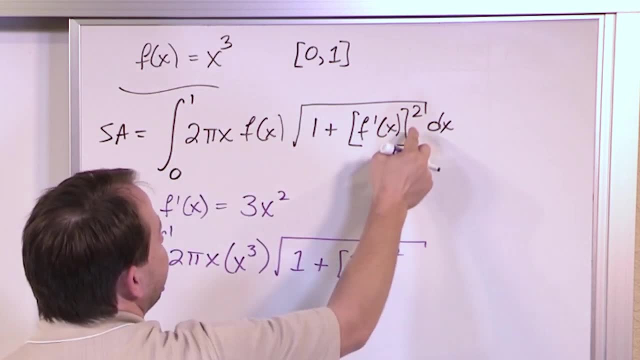 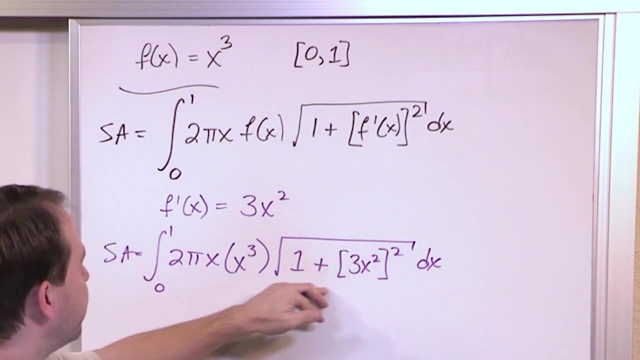 times the square root of one plus three x squared, because that's the derivative and that quantity is squared. So we take the derivative of our function, we're squaring this quantity and this is all under the radical dx. So I'm spelling everything out. I'm not really oversimplifying. 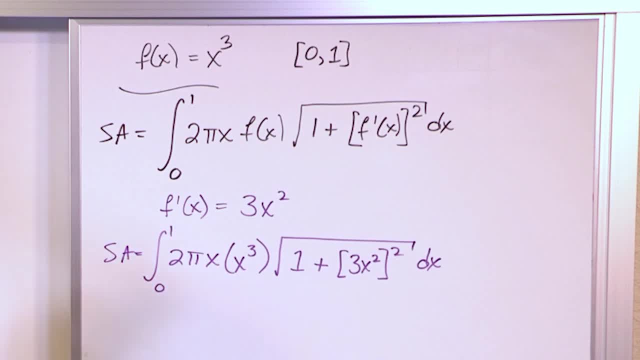 I'm putting what f is, I'm putting what the derivative is and it's spot. and I'm going to do simplifications on the next step so that I don't get myself into trouble. So what I'm going to have then, I'm going to take the two pi out integral from zero. 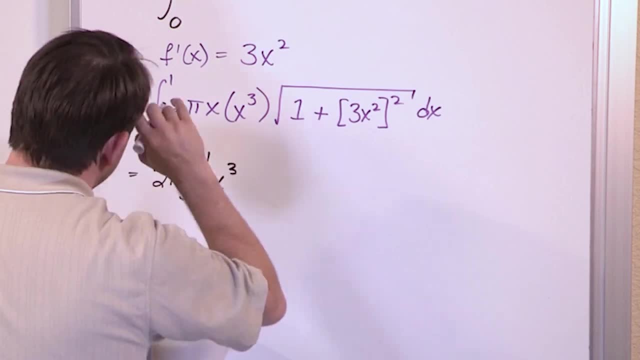 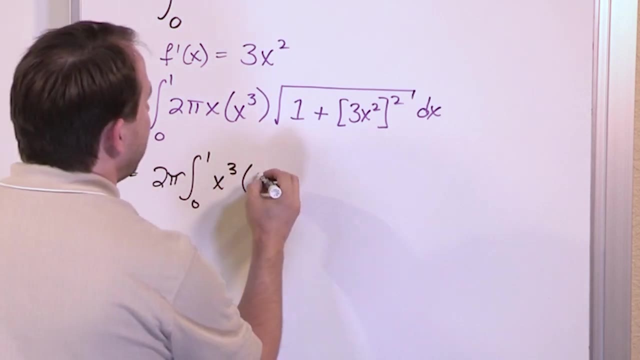 to one, and I'll have x cubed here, And then what I'll have here is, instead of a square root, I'm going to change it over into a fractional power, So I'll have one x squared And then I'll have x squared. 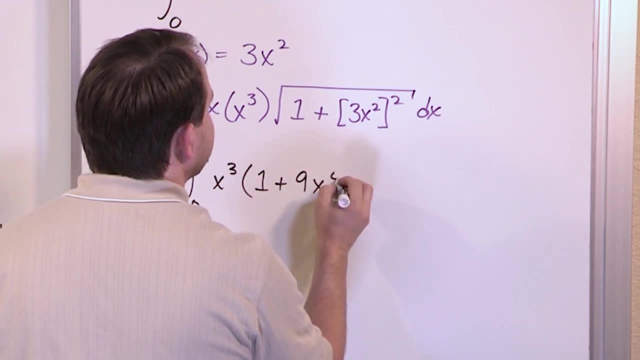 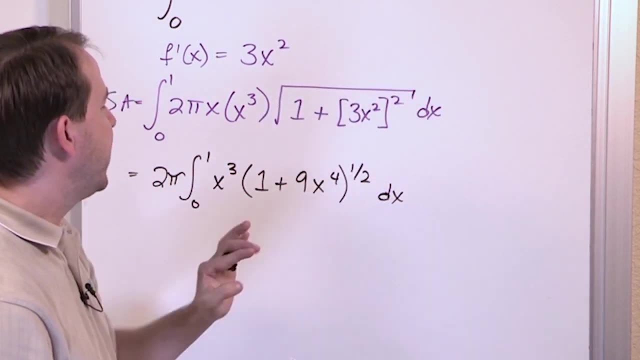 One plus three squared is nine. then x to the fourth power and this is one half dx. Make sure you understand that. All I did is I changed the square root into a one half power because I like looking at that instead. It's just a personal preference. 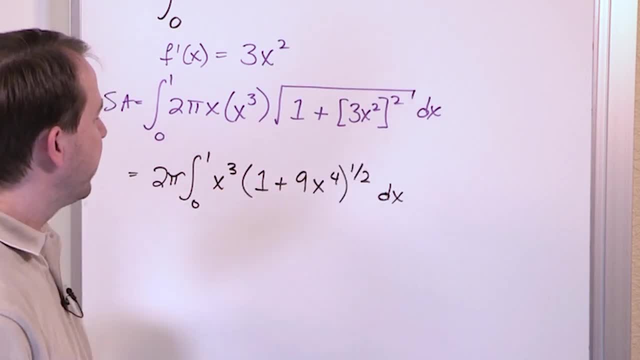 One plus stays the same. Squaring, this quantity gives you nine x to the fourth power. So I'm done. Now I need to figure out a way to integrate this guy. Now you know, when you have things under a radical it's kind of a huge clue that you're 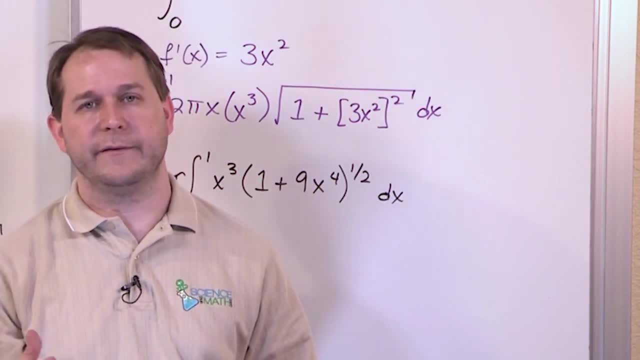 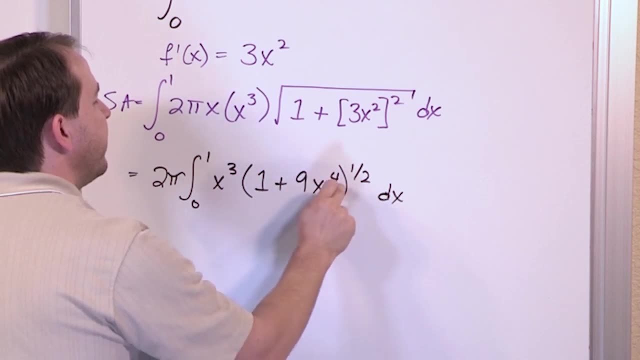 probably going to need substitution somewhere along the way, Almost always. And if you look at this and you say, well, what if I choose this inside of the radical as my u, then the derivative of this quantity would be 36 x cubed. 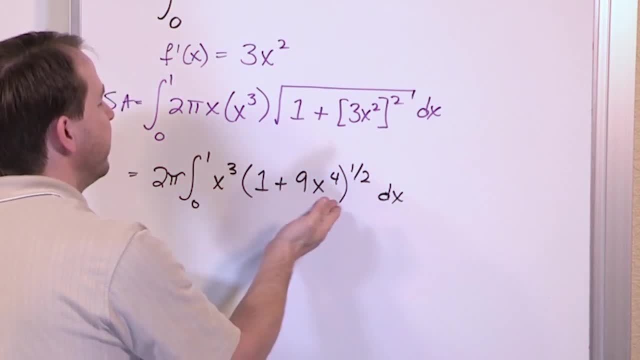 And we know that in the end we've done enough of these, that whatever this derivative is of whatever u ends up being is going to be on the bottom. So the x cubed should cancel with what I have out here. But you know, even if you don't see that ahead of time, it's probably a pretty good bet that. 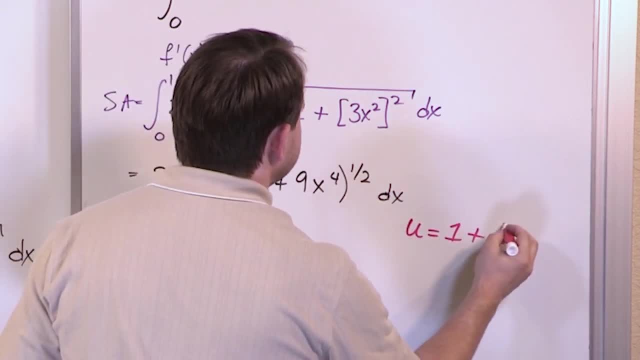 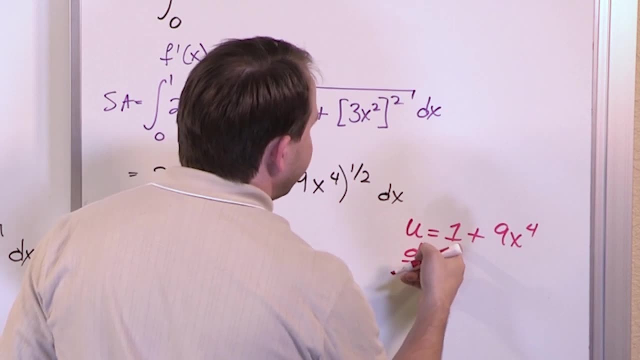 this is going to be the correct u: One plus nine x to the fourth power, One plus nine x to the fourth power, One plus nine x to the fourth power. So that would mean du dx Derivative of this is zero. Derivative of this would be 36 x cubed. 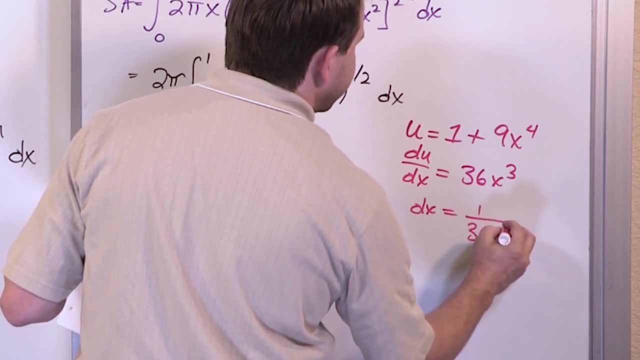 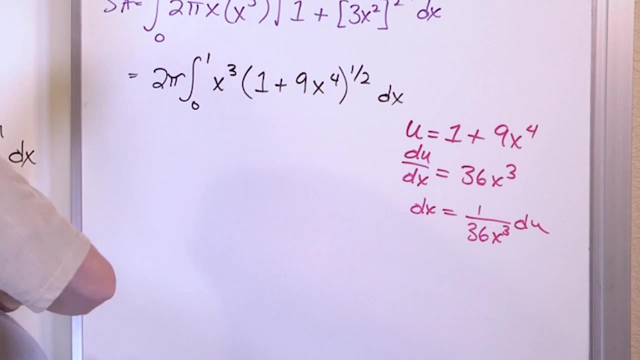 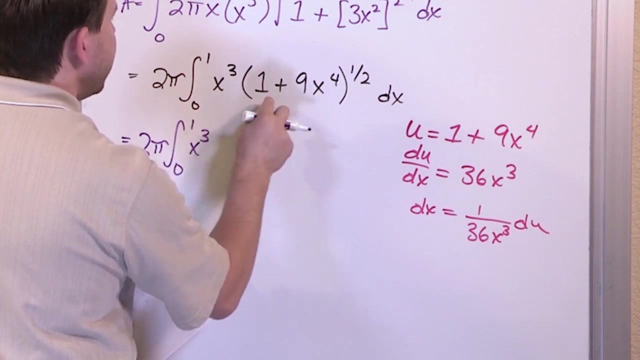 So that dx would be one over 36 x cubed du. So hopefully this x cubed will cancel with the ugly one that we have preventing our integration. So we have two pi integral zero, one x cubed. This whole thing is u. 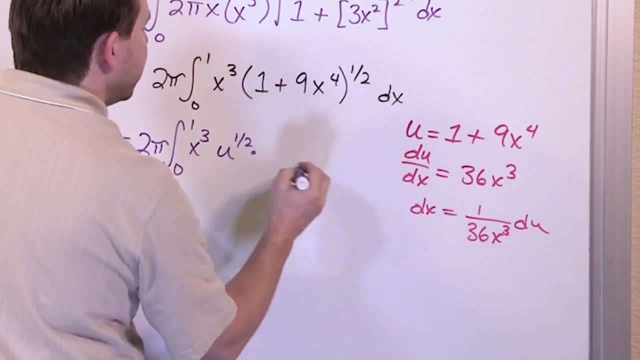 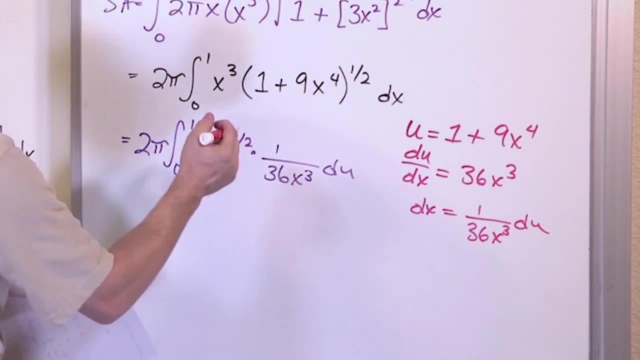 We've defined it So u to the one half And then dx. we know what that is: One over 36 x cubed du, And if we've done everything right, then we have x cubed canceling with x cubed. 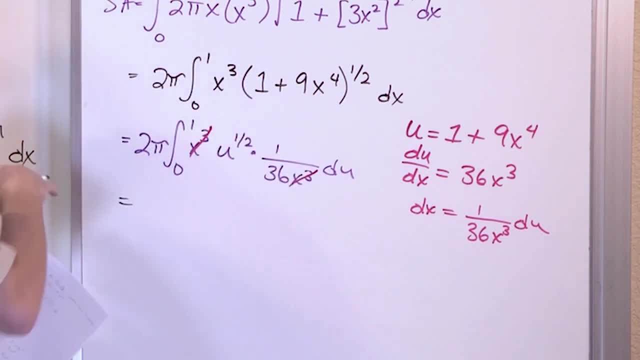 And so what we're going to have. then the one over 36 can come outside the integral, And so what you're going to have. you have a two already out here. You take a one over 36 out, So two over 36 is going to be one over 18.. 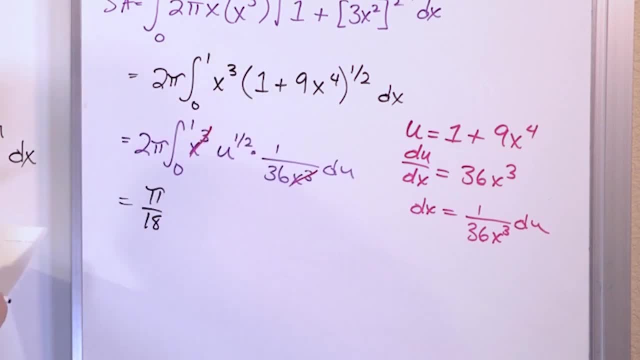 So what you're going to have is pi over 18.. Outside the integral, That's just from taking the one over 36 out Integral zero to one, u to the one half du. That's a super integral, super simple integral that we know how to solve. 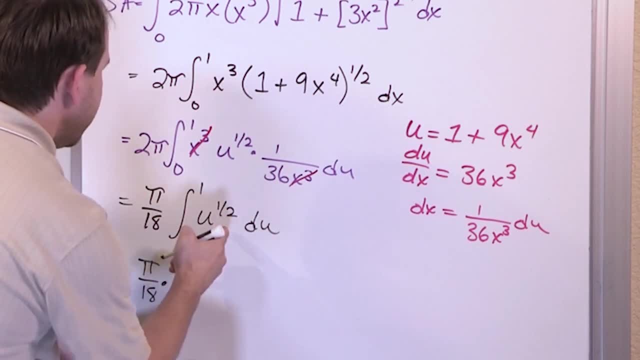 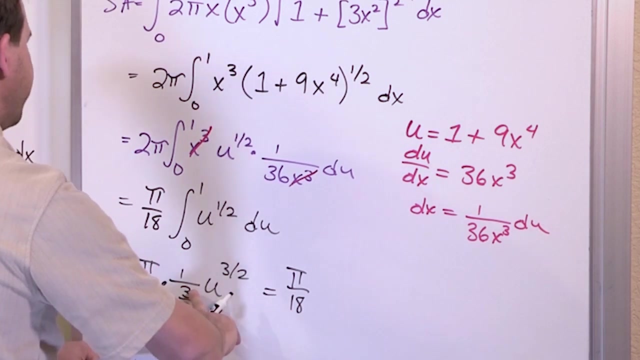 So what we get is pi over 18,, right. And then we just do this: One over exponent plus one is three halves u to the three halves, right, And that's going to be. what we have is pi over 18.. And then three halves. we can flip it over and multiply, so we're going to get two thirds. 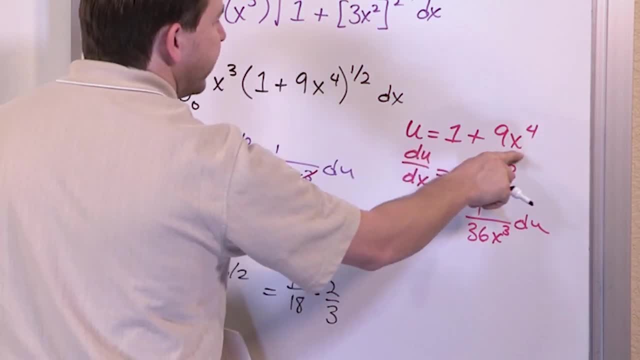 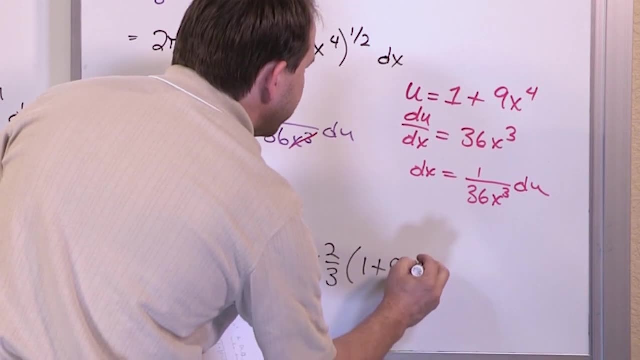 And u, since we know what u is equal to this guy, we're going to stick it right back in. So it's going to be one plus nine to the fourth power, nine x to the fourth power, And we're evaluating this whole integral from zero to one. 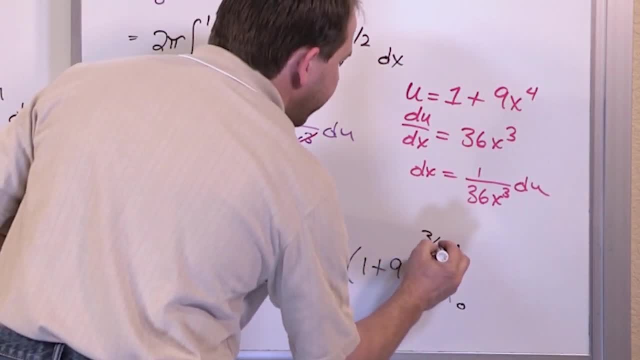 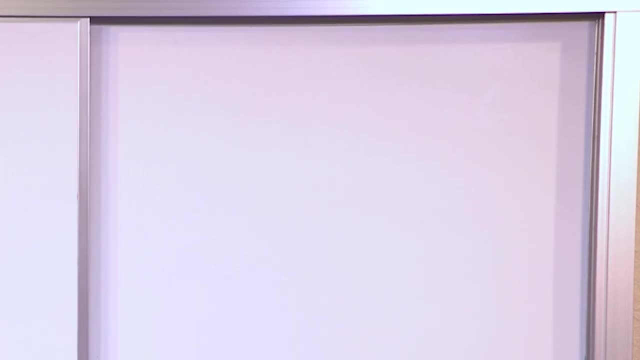 And this u that we put in here, don't forget, it's to the three halves power. So three halves power. So this is what we have to evaluate from the upper and the lower limit of integration. Now, all I'm going to do here is notice when I go over to the next step that I have. 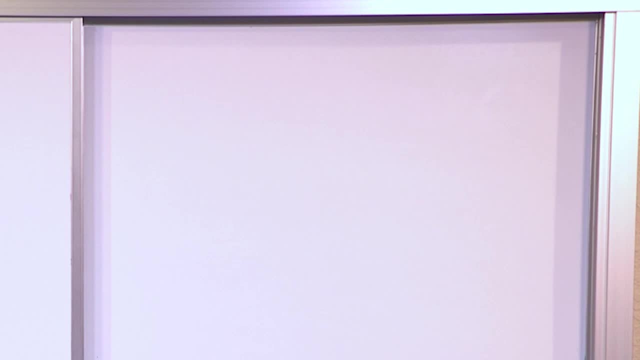 a two and an 18.. So that's going to give me a nine down here, And nine times three is actually 27.. So really all I'm going to have out here is pi over 27.. And on the inside I'm going to have one plus nine x to the fourth power, all raised to: 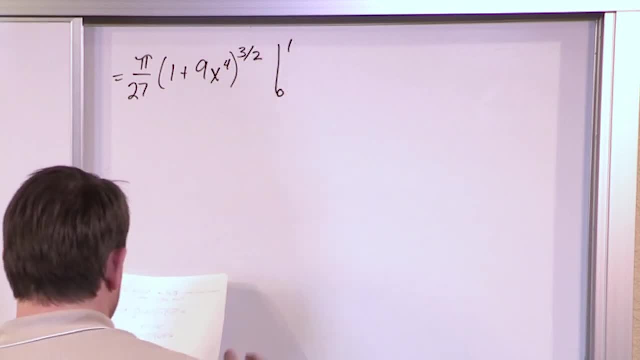 the three halves power, And that's evaluated from zero to one. All right, So I've evaluated from zero to one, And I know that I can crank through this by saying pi over 27. And I'm plugging in a one here. 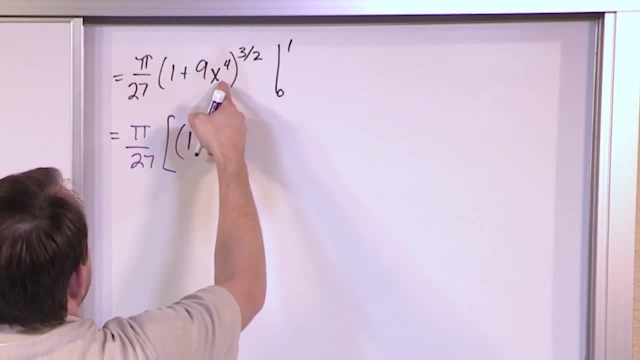 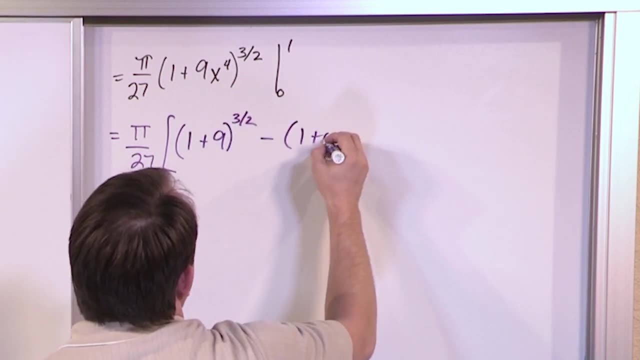 So all I'm going to have is one plus nine, because one to the fourth power is just one. So one plus nine to the three halves, And here I'm going to have one plus zero to the three halves. Make sure you understand that. 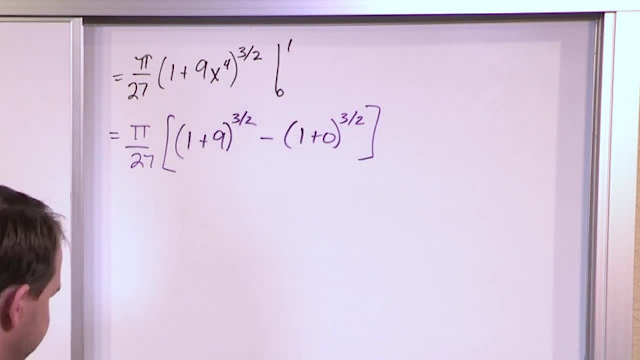 Because when I put a zero in here, it just gives me zero. When I put a one in here, I just get this nine. So really all I have is pi over 27 times 10 to the three halves, And this guy is going to be minus one. 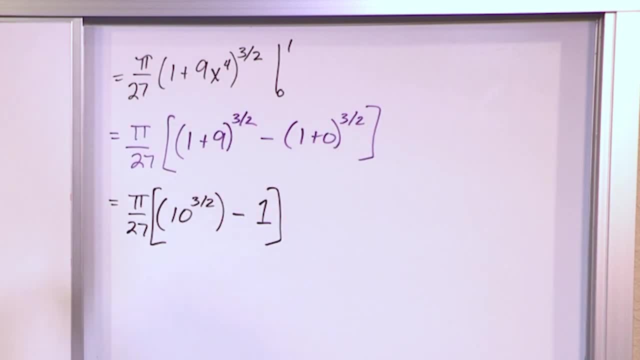 Because one to the three halves is just going to give you one, And this is the final answer: Pi over 27,, 10 to the three halves minus one. You could do some business here. You could try to simplify a little more. 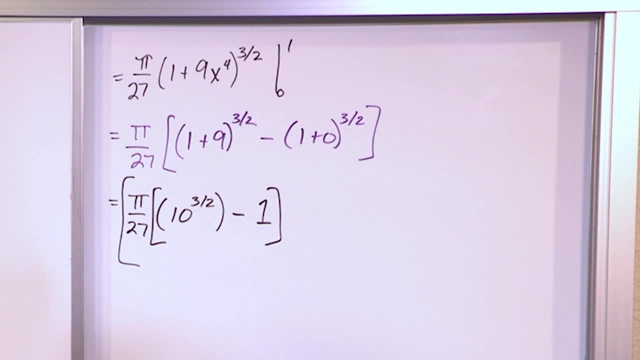 But ultimately it's not going to get much simpler than what it is right here Other than just going to a decimal, And you could probably do some other things and make it look different, But this is basically going to be the final answer. 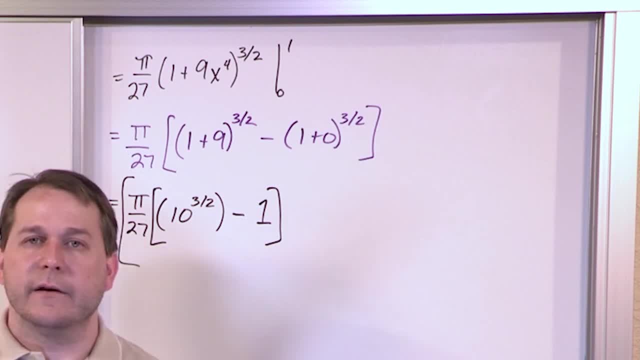 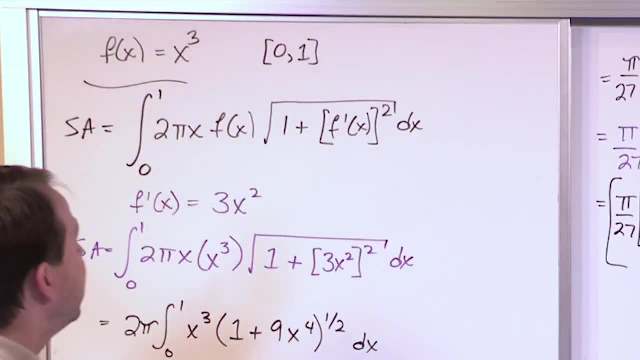 And what would the units be? here? The units is going to be units of area, So it's going to be square centimeters or square meters or square inches, or whatever you're working with Depends on what your original problem was. 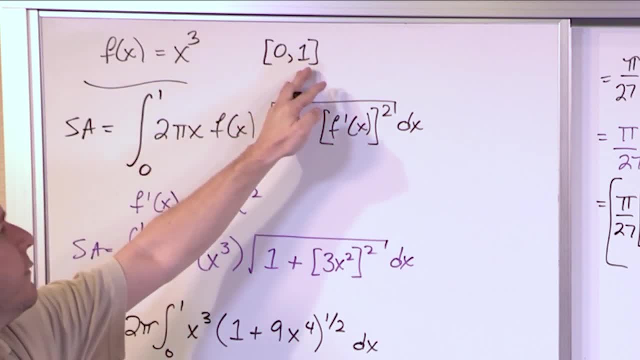 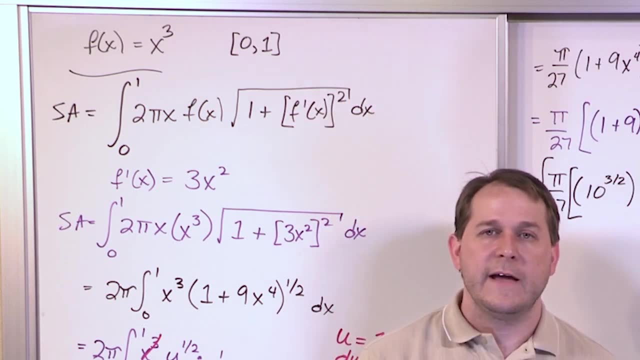 When we said our original function was x, cubed over the extent from zero to one along x. if we're measuring the extent of our function in centimeters, then that means that the answer we get is in square centimeters. If we're measuring the extent of it in centimeters, then that means that the answer we get is: 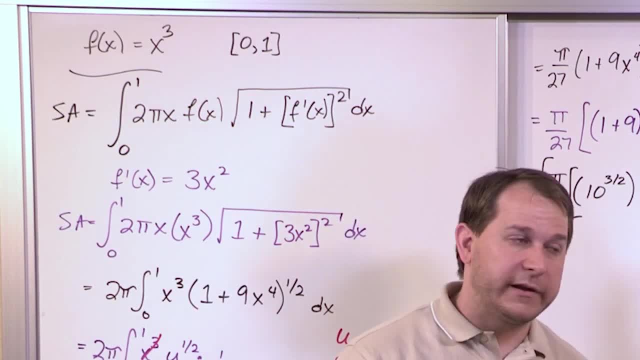 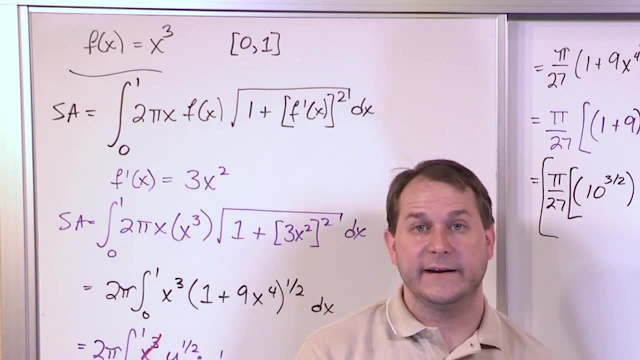 in square centimeters. If we're measuring the extent of it in kilometers or something, then it'll be square kilometers. But what we've done is we've found the surface area of this curve between this boundary revolved around the x-axis. 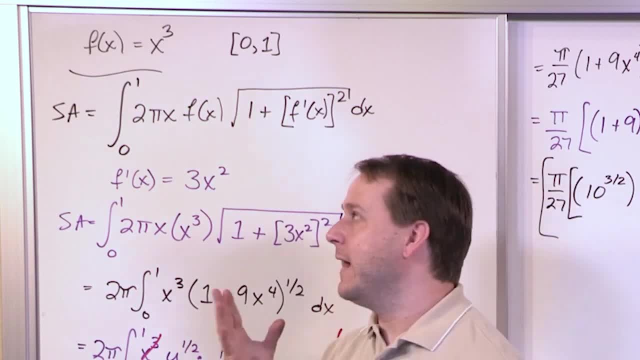 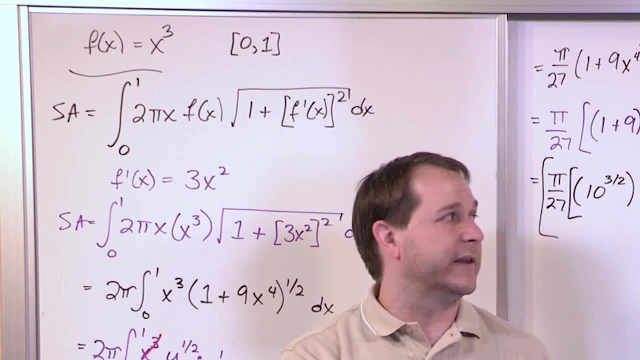 So you just have to follow the directions, so to speak. You have to take the derivative, then square it, then add the plus one. You need to do everything in the proper order, Because if you don't do that, then you're definitely going to get the wrong answer. 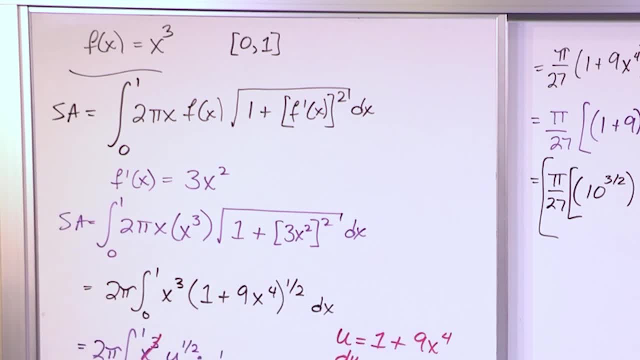 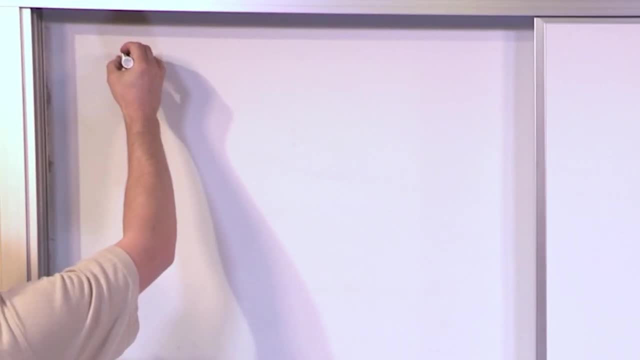 So let me go and erase this board And I'd like to do one more problem of surface area, just to give you a little more practice. All right, the next problem is kind of interesting, I think, because it makes you forces you. 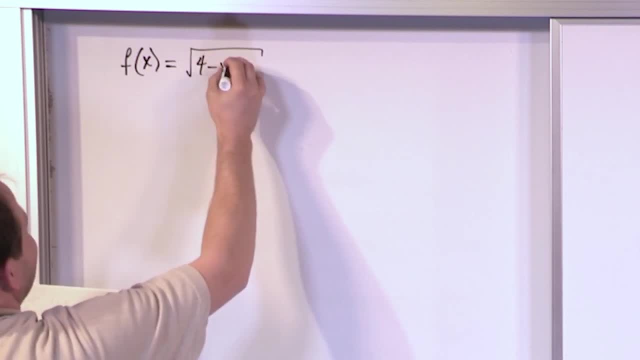 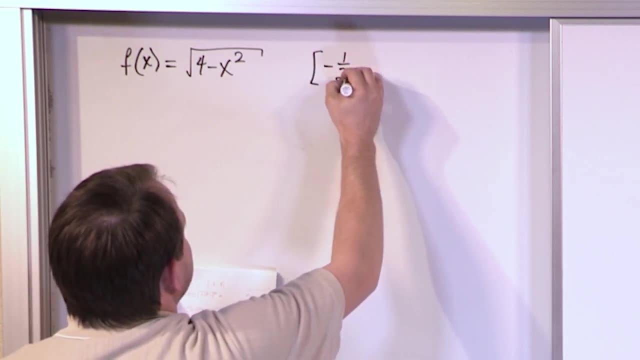 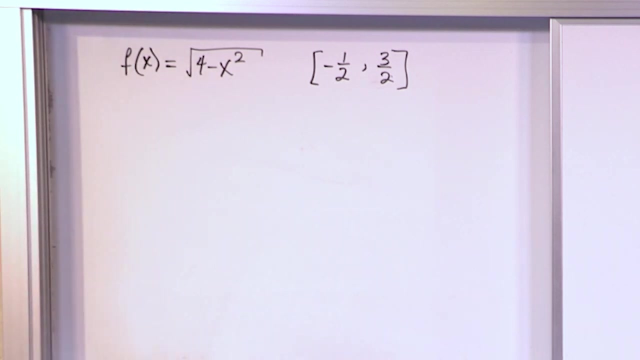 to be careful. Square root of four minus x squared. that's our function, And the extent along x that we're going to look at is from. x is equal to negative one half to positive three halves. So what this means is if you plot this function and then you only look in the region between: 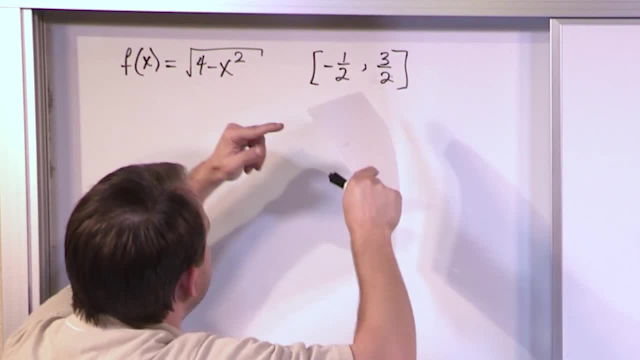 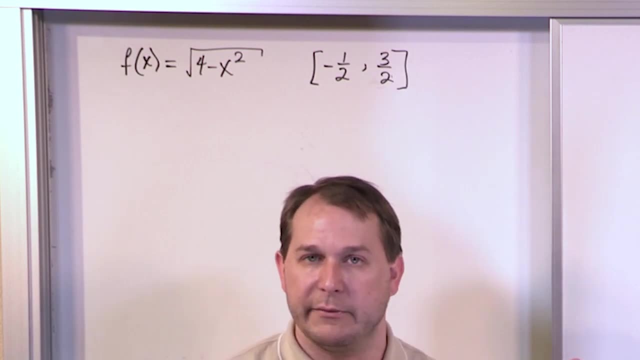 negative one half and positive three halves and kind of chop that function at that point and you revolve that function, whatever it looks like, around the x-axis. we want to find the surface area of the resulting revolution that we have. So we just sort of follow what we know. 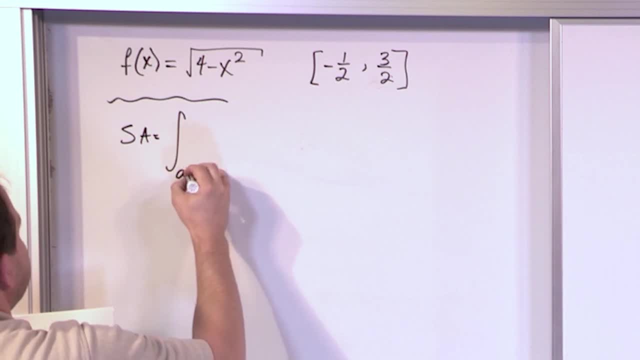 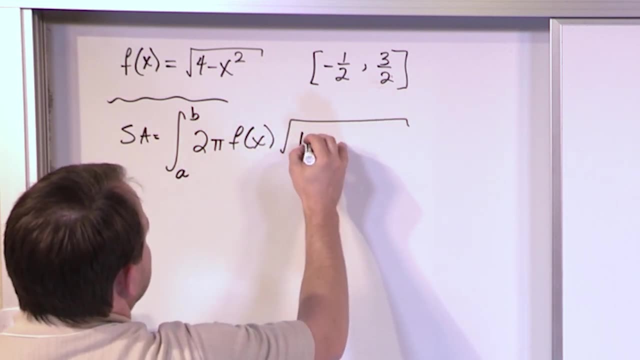 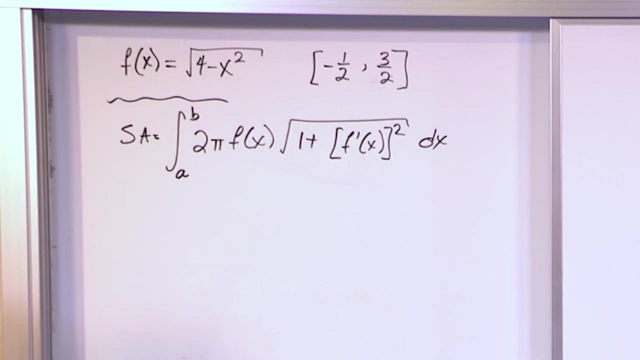 We know the surface area is going to be the integral from a to b. We know what a to b is: Two pi f of x, square root, one plus f prime of x. Okay, And so what we need to do first is find the derivative of this guy. 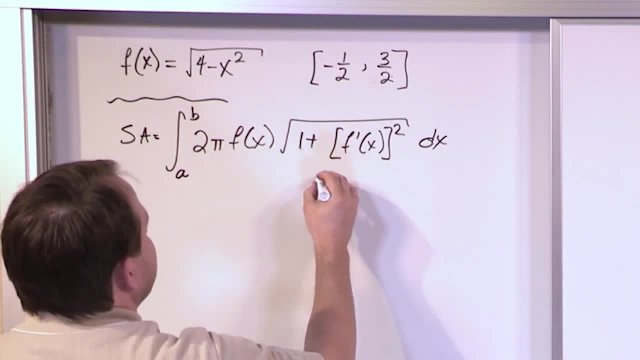 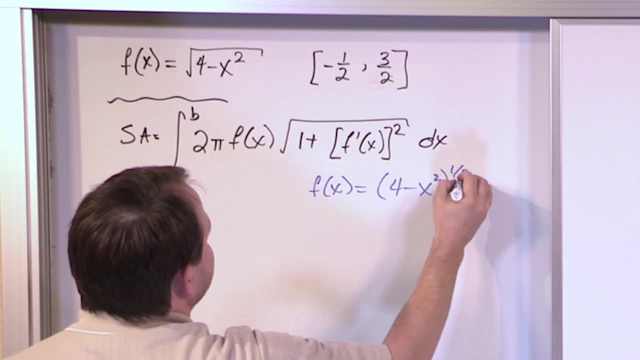 So f of x, we already know, is equal to this, but I want to write it as four minus x, squared to the one half, because it helps me take derivatives. F, prime of x. how do you take the derivative of this? 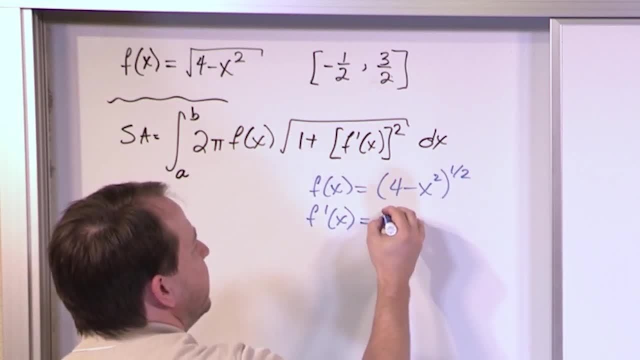 This is the chain rule, right, Because we've got with square root, we've got something inside. So it's one half Four minus x, squared to the negative one half, because we're taking the exponent minus one. Then we have to multiply by the derivative of what's on the inside. 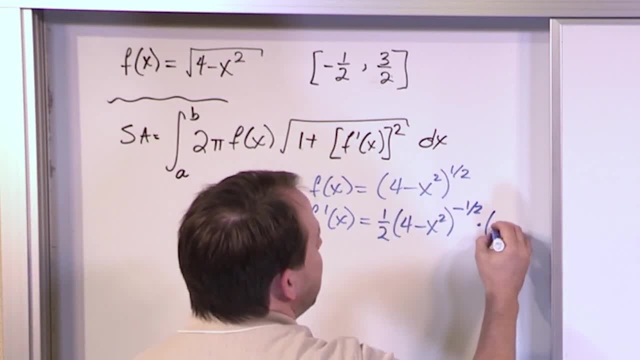 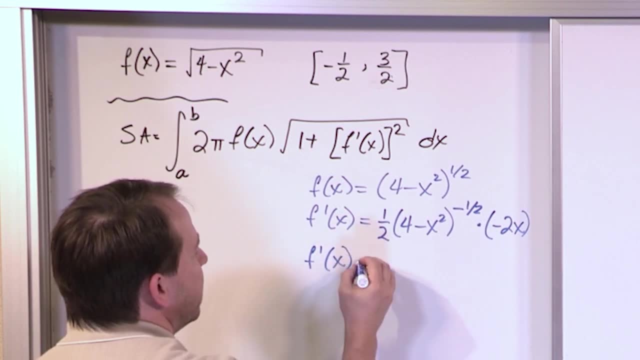 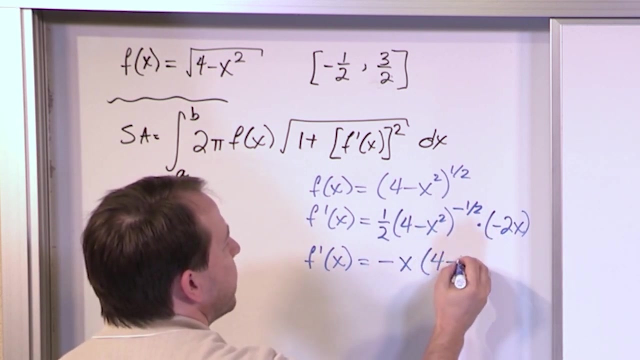 So the derivative of four is zero. The derivative of negative x squared is negative two x. Okay, So that's how you take the derivative there. If you need practice with that, go take a look at our derivative examples. The one half and the two are going to go away, so you're still going to have a negative x. 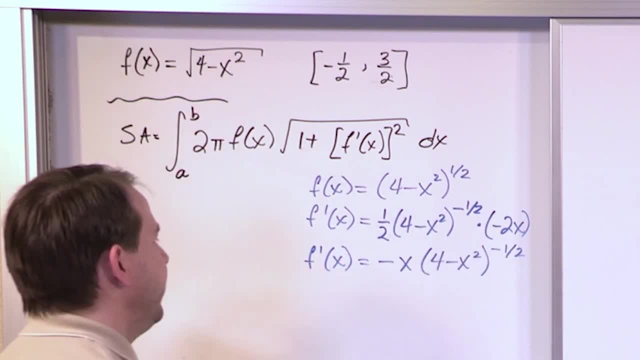 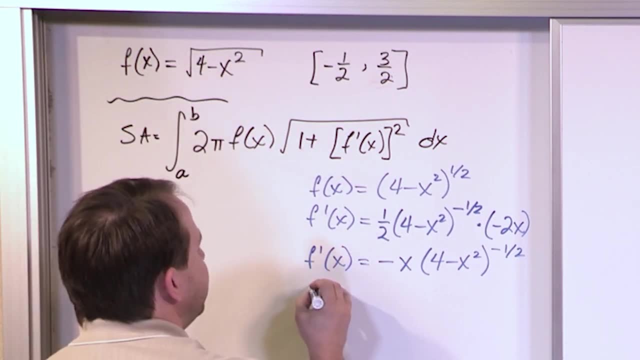 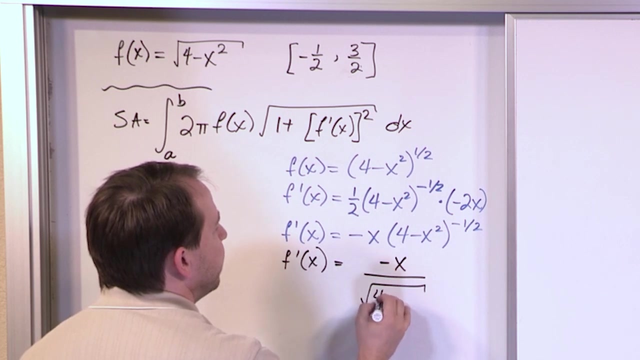 Four minus x squared to the negative one One half. And since our original problem is in terms of square roots, I'm going to go ahead and choose, not required to turn it back the way we were given the thing. So we have negative x over square root. four minus x squared. 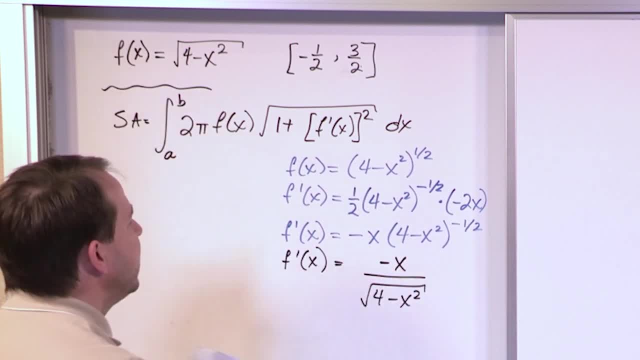 It's on the bottom because we have a negative one half, so we can write it like this: You can choose to plug this into the problem or you can choose to plug this version into the problem. They're both exactly the same thing, so don't stress out on which way you choose. 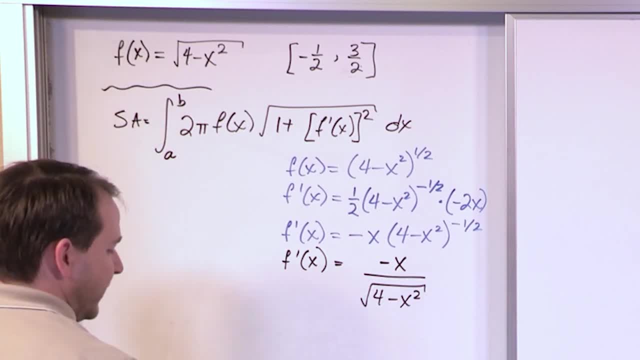 It's just the same sort of thing. It's just the same sort of deal. So we're finally to the point where we can plug in something. So the surface area is going to be the integral from a to b. but we now know that that's from. 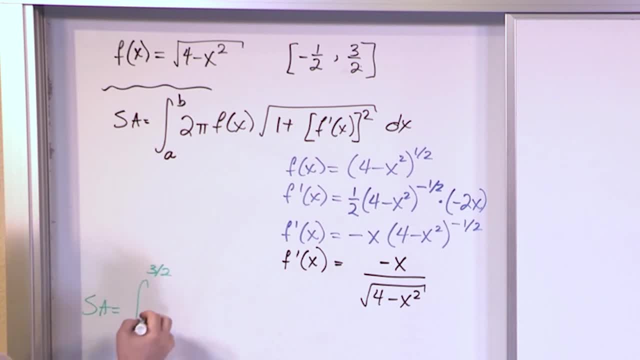 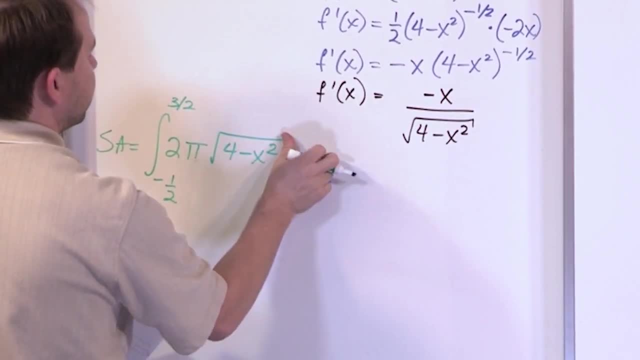 negative, one, half up to three halves, Okay. And then we have two times pi, times f of x. F of x is four minus x squared Right. And then we have this other big radical, So we have another radical right next to it. 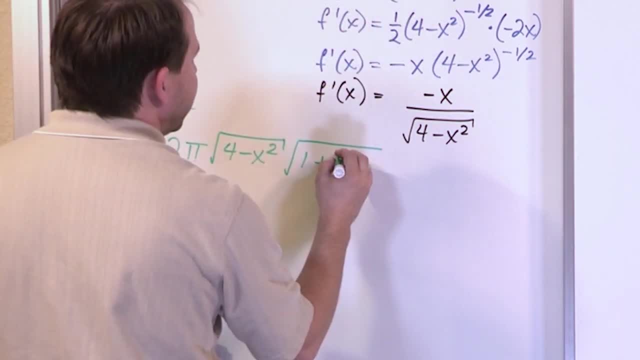 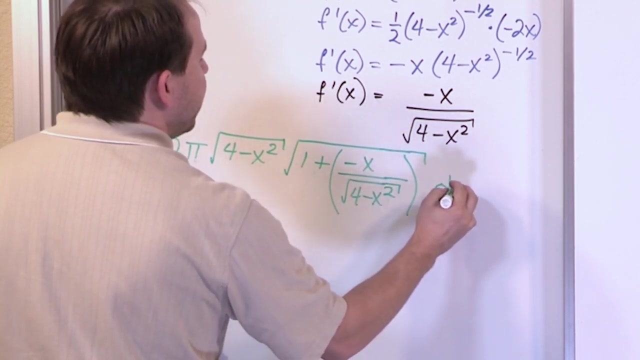 One plus and then we have this guy. just to make it totally clear, I'm going to open a bracket. The derivative is negative x over square root, four minus x squared. Close that inside, radical there. Close this guy here and then bring this guy here, dx. 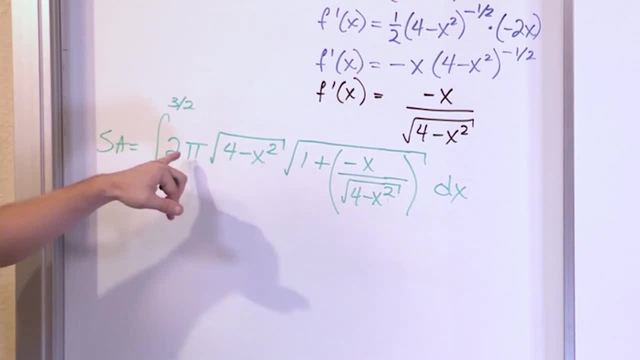 This is absolutely atrocious looking. I mean, you have four minus x squared out here under a radical, and then you have a radical here and you have one plus this guy. Now this derivative. I even forgot to put a square here. That's essential. 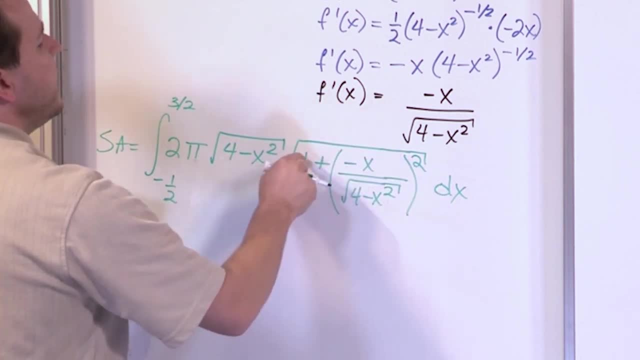 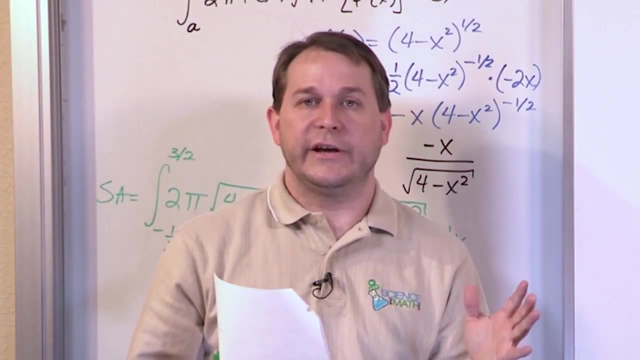 So what we have is the derivative of our function. inside here This is going to be squared. Then we have to add one. We have these square roots everywhere. When you get to this step in a problem, you start to get worried because you feel like 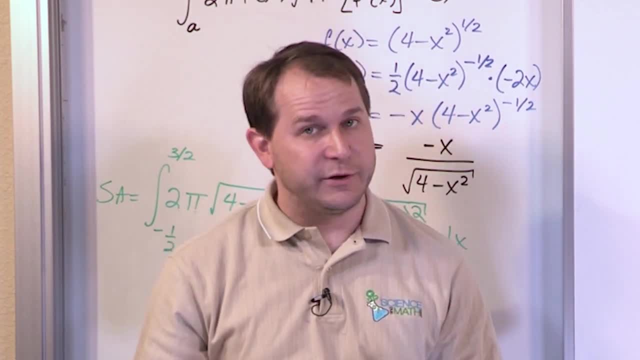 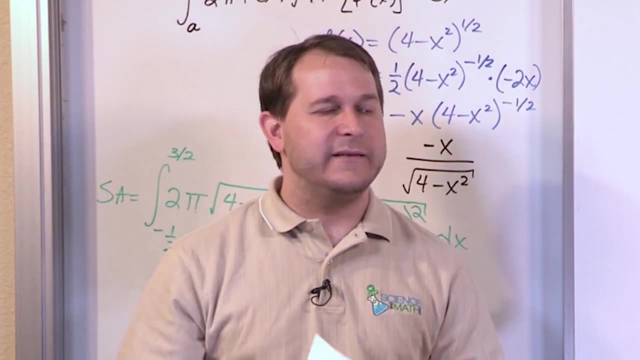 how am I going to integrate that? I have no idea. Well, what I was trying to tell you before is these problems. they have to fall out so that what you get at the end is easily integrable, Easily able to take the integral of. 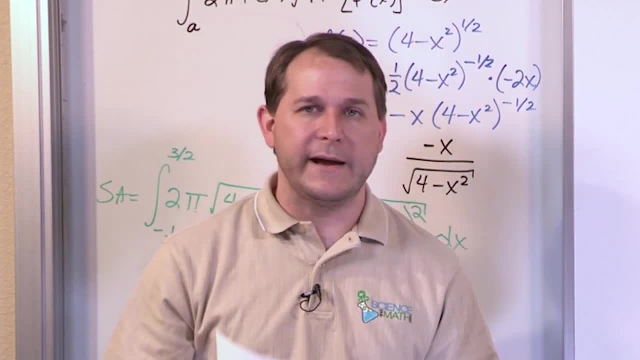 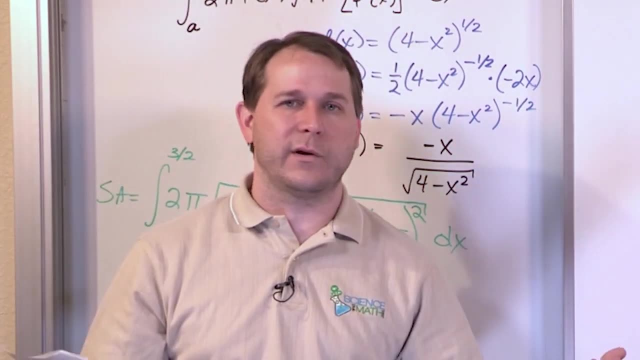 If you're not able to do it, If you can't simplify it, If it's something that looks simple, then you've made a mistake somewhere or you're just setting it up wrong, Because if you stick any arbitrary function into this, if I just pick secant squared of 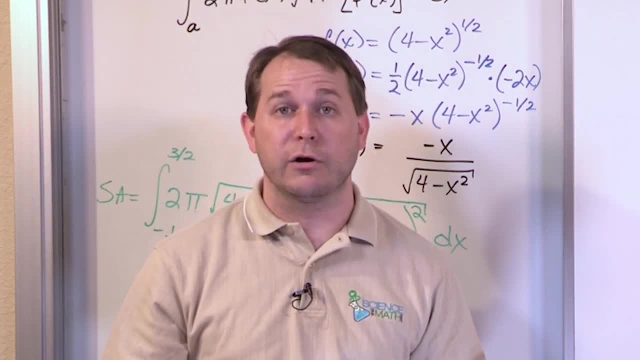 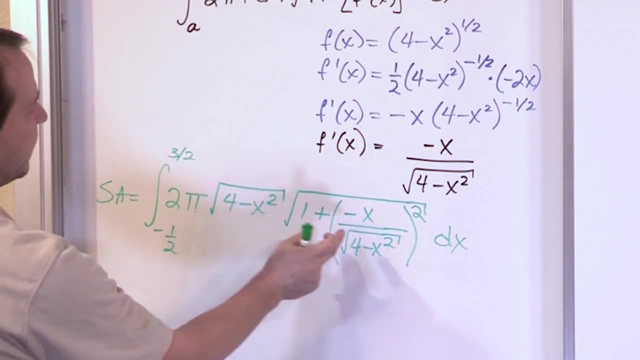 x and stick it in there as a function, you're going to get crazy intervals that are going to be hard to solve. So anything you see on a test should resolve down easily. Now we see we have a four minus x squared. We see we have a four minus x squared. 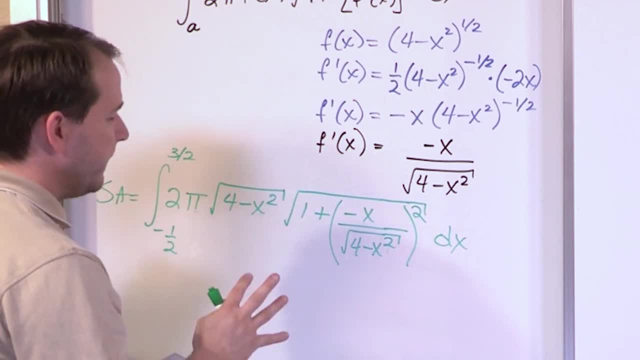 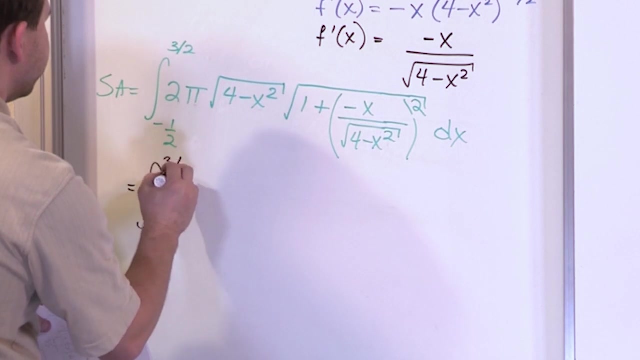 Maybe that'll help us, But what we know from our immediate work is that we need to square this and then we need to add the plus one and everything else. Maybe, if we're lucky, we will get something nice. So what we have is the integral from negative one half up to three halves, two pi four. 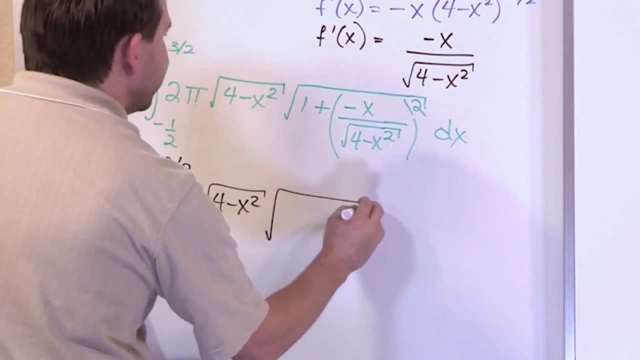 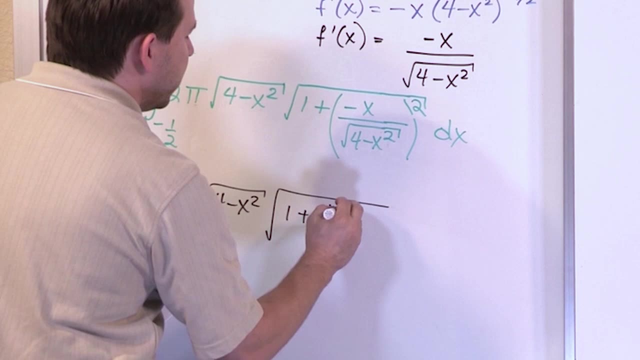 minus x squared, And then inside here we have one plus. Now here's where things get interesting. We square this whole quantity, So on the top it's going to be x squared, Because negative times, negative- is positive. On the bottom you're squaring a square root. 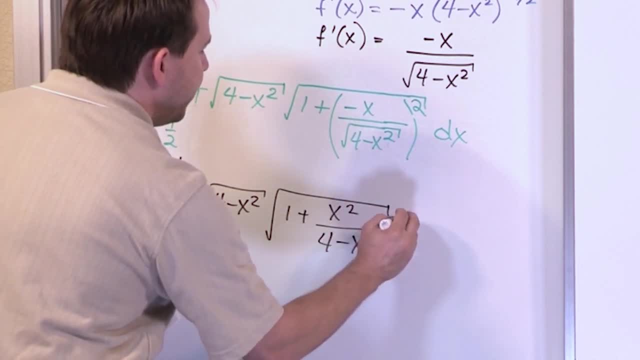 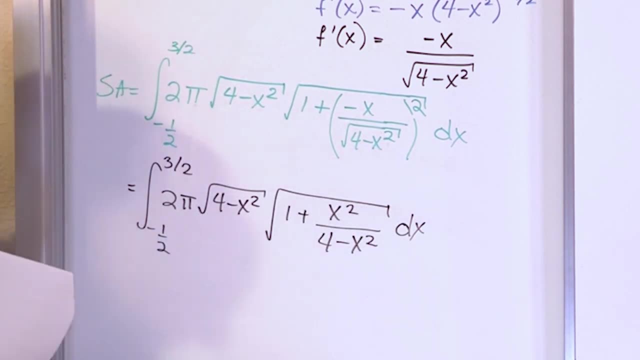 So really all you have on the bottom is four. So you're going to have a four minus x squared dx. Now you're getting to a point where you kind of have to be a little creative. You need to decide for yourself which way to go. 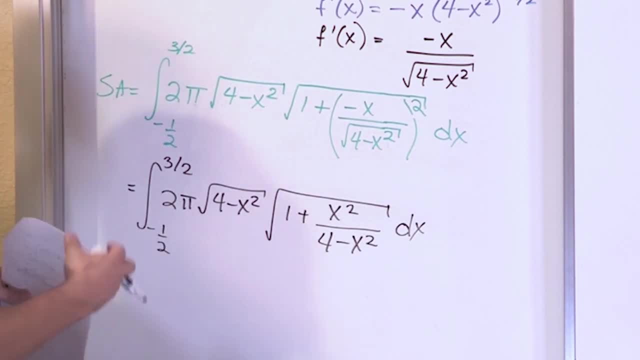 And things can be not as easy as they can seem harder than they are. What we have is one plus this quantity. This is impossible to really add together. We can't just add one to it and do anything simpler, because you have a one out here and 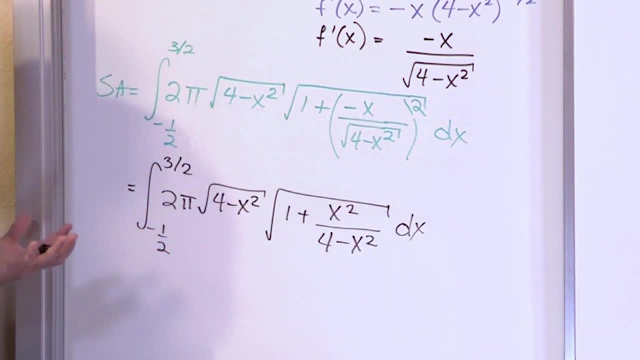 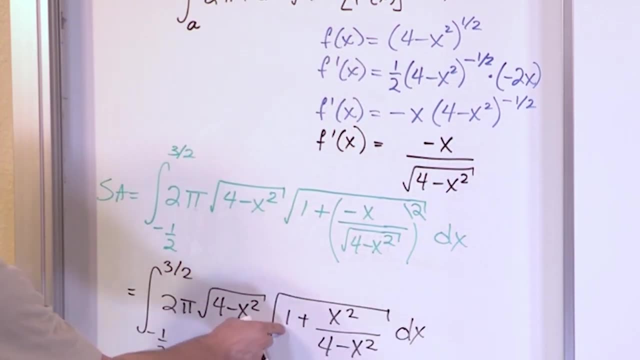 you have a fraction here, So there's a couple different ways you can go, But the thing that jumps out at me is that when you're adding one to any quantity, it's very easy to add one, Because the way I'm going to write this one in the next step is I'm going to write this: 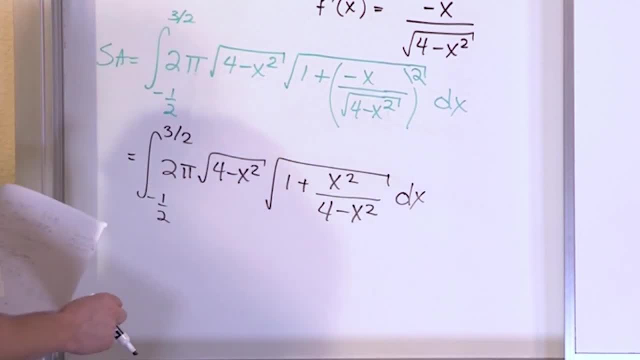 as four minus x squared over four minus x squared. And if that doesn't seem right to you, just think to yourself. what you're trying to do is find a common denominator to add these together, And that is something you do constantly. whenever you're doing that, 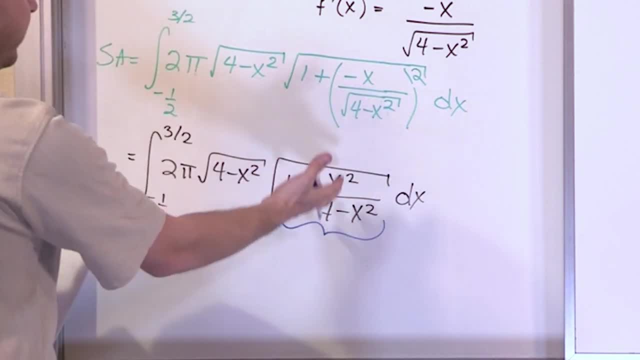 So if I do this, let me just work on this, And, by the way, I do this on my paper a lot, you know, even when I was in school. So I'm going to start with this point. and then you draw a little bracket and say, okay. 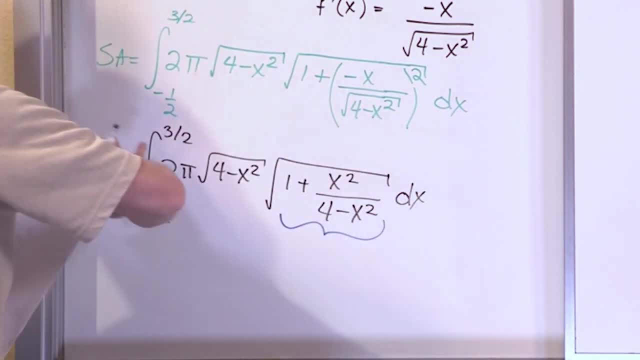 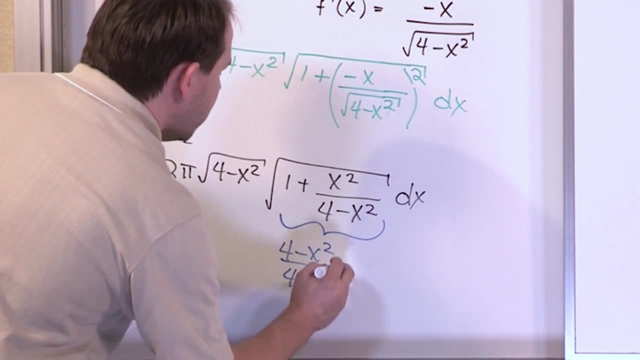 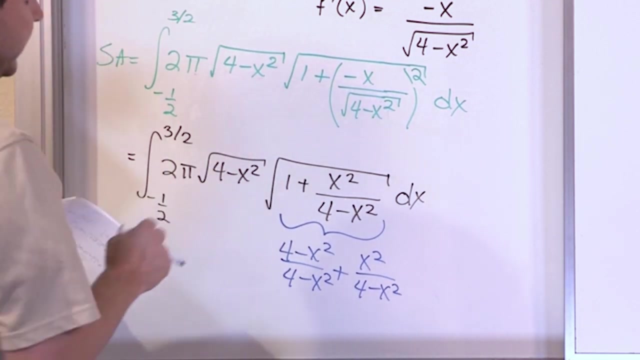 I'm going to work on this So you don't have to keep writing the whole problem over and over. So what this will be equal to is four minus x squared over four minus x squared, plus x squared over four minus x squared. I mean, all we've done is taken the one and we've made it as a common denominator, because 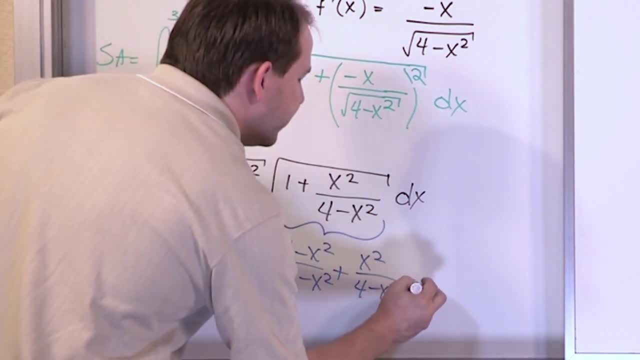 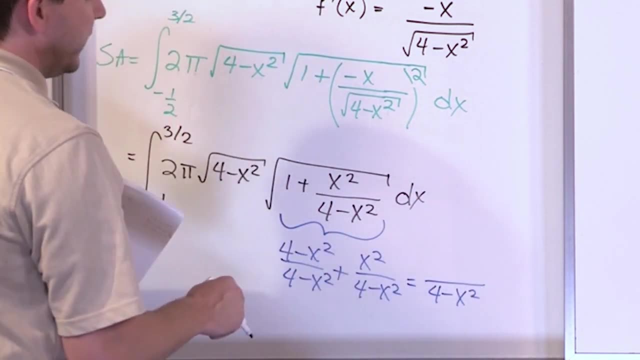 anything over itself is one. So when I do this, I see that my denominator is going to stay the same: four minus x squared right. Four minus x squared, plus x squared. So really that's my new numerator, And this looks significantly simpler than what I actually had in there to begin with. 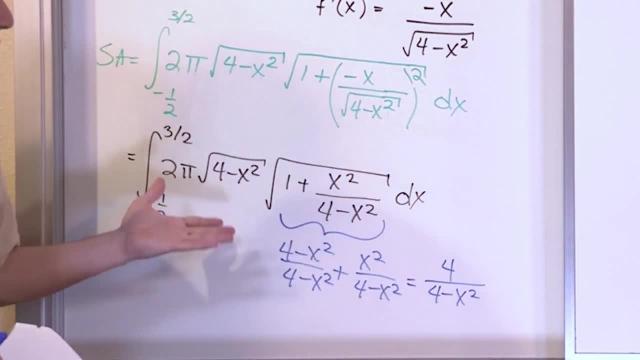 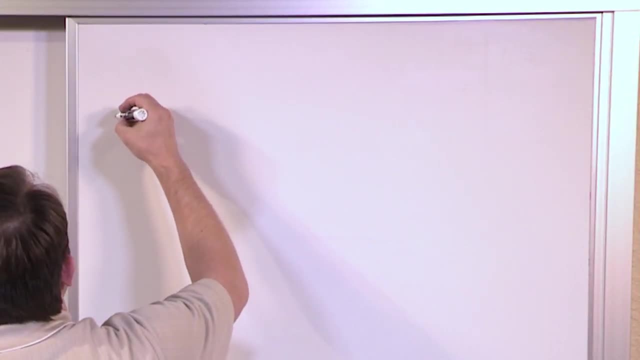 And it's not magic, It's not a math trick, It's just getting a common denominator between these two. So let's go and rewrite the integral on the other board and continue working. So what we have is the integral from negative one half up to three halves of two times pi. 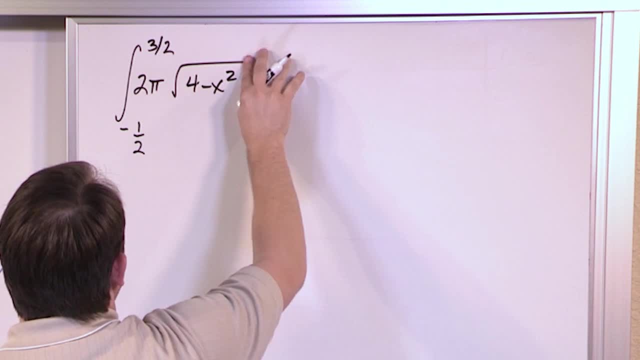 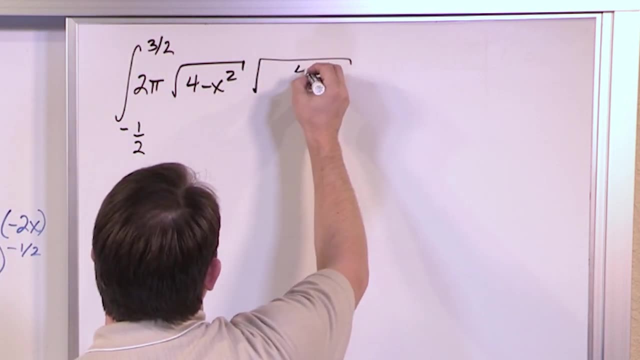 And I still have my four minus x squared. So I've got my four minus x squared under the radical there, And what I have? I have another radical, but now I have four over this, So I have four over four minus x squared, dx. 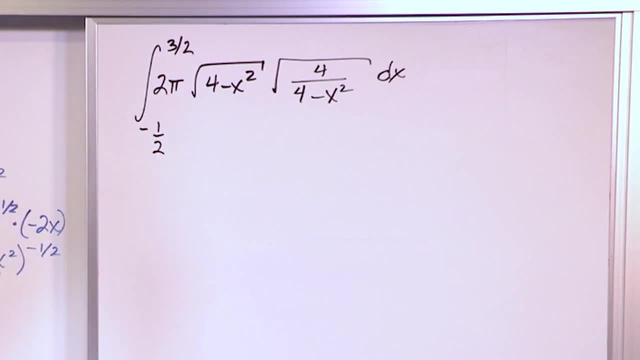 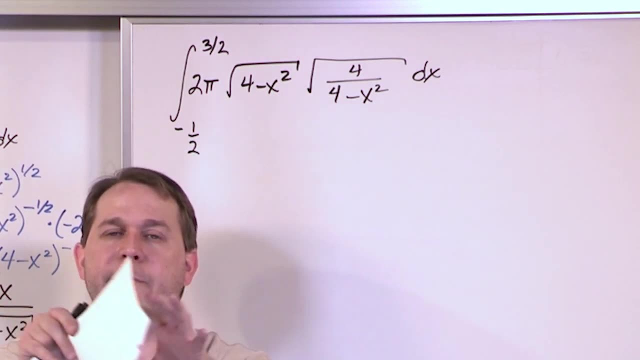 So I have to solve this integral. Things are getting a little bit simpler Now. you guys should all remember: when you have a radical multiplied by another radical- like a square root times a square root- what you can do is merge them into one common entity. 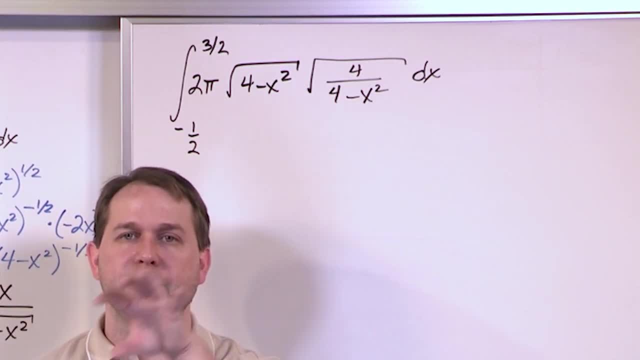 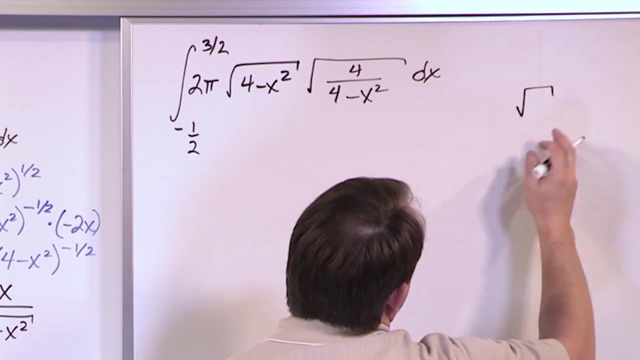 All you have to do is combine them under a single radical, But you have to multiply the insides together. So, in other words, thinking back to algebra, just to kind of prove it to you a little bit, square root of you know, I don't know- nine times the square root of nine. okay. 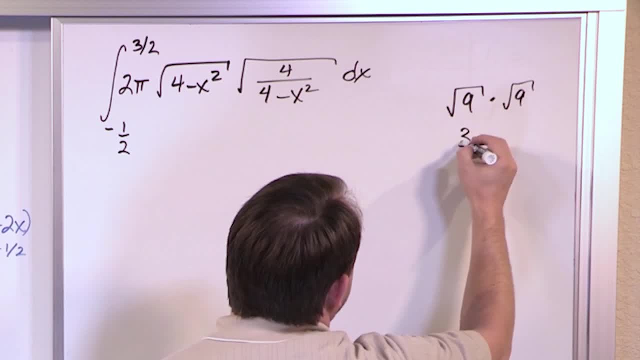 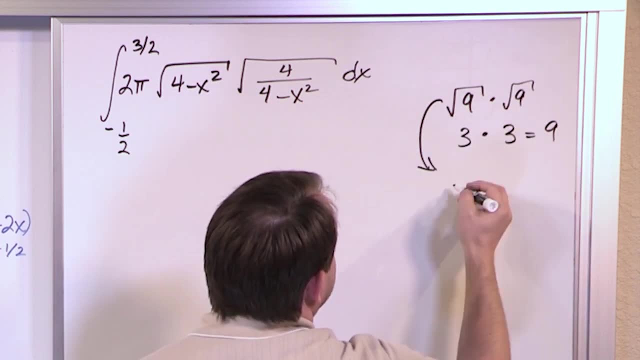 How would you do this? Well, the easiest way to do this, you would say: the square root of nine is three. The square root of nine is three. So the answer you get is nine. But another way to simplify this is: when you have a radical times a radical, you just take 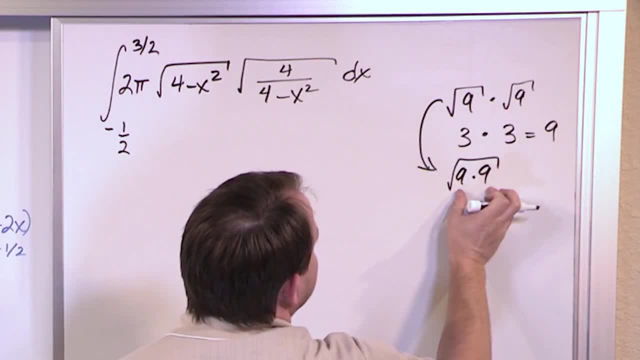 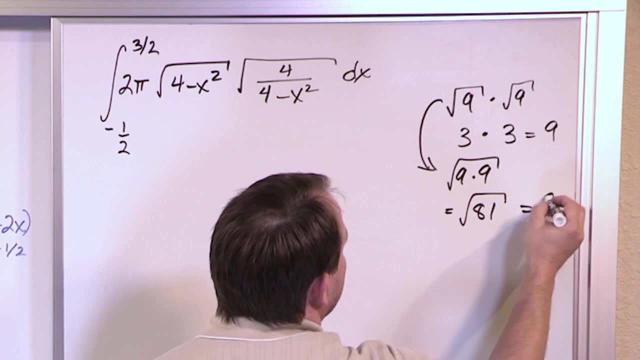 and you do the nine times nine on the inside, And you take the insides, You multiply them together And you combine them under a single radical. So what you're getting is the square root of 81, and the square root of 81 we all know. 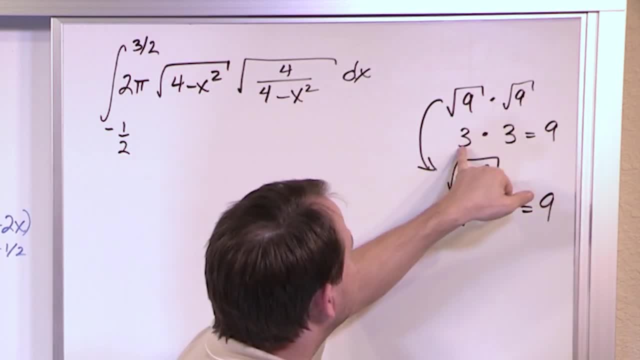 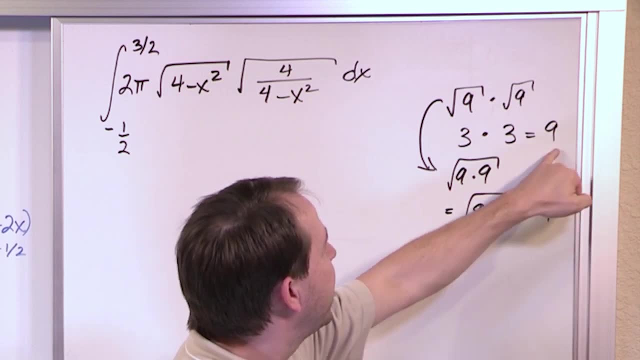 is nine. So whether or not you simplify the radicals ahead of time and multiply the answer, or you just combine them under a common radical by multiplying the insides and then simplify, you're getting the same thing either way. I'm just proving that to you, if that's something that you don't remember. 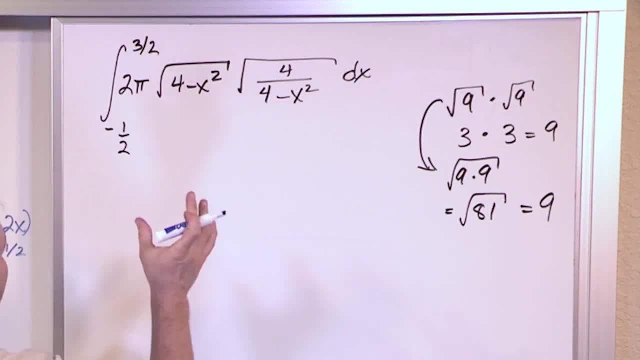 Because you know you do forget things over time. Everybody does So. what this means is I can combine these radicals together. So I've got negative one-half, three-halves, and this is going to be one giant radical where I'm taking this and multiplying it by the inside. 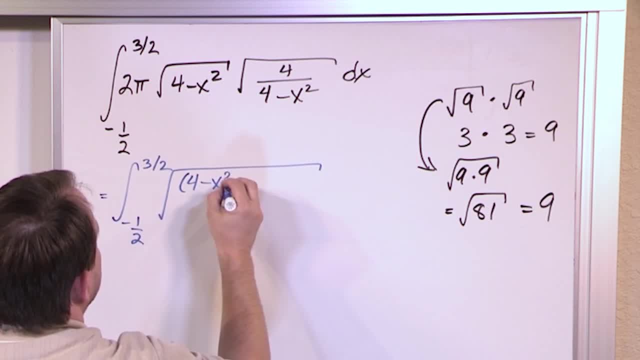 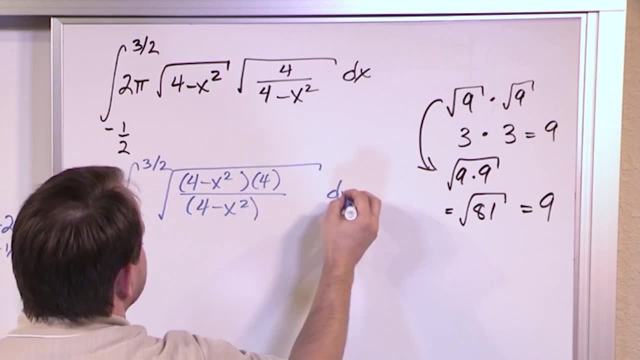 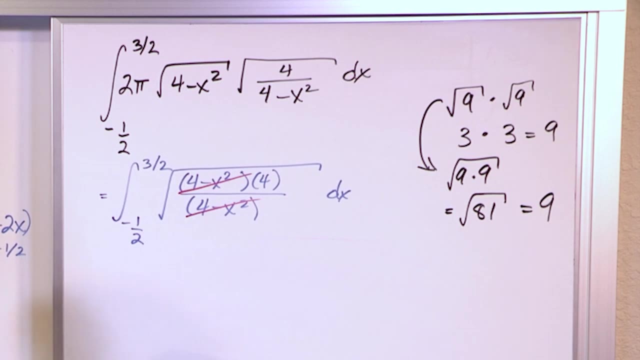 So I'm going to have four minus x squared times four on the top. I'm going to have four minus x squared on the bottom. Now you can see how this problem was specially constructed, because that disappears. And not only does it disappear, what I'm left with is the square root of four. 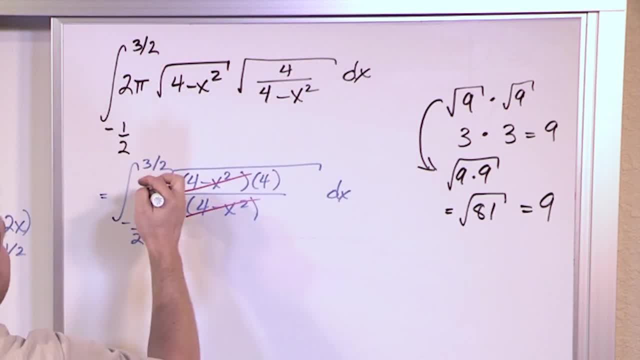 So I've got negative one-half, three-halves, and this is going to be one giant radical with is the square root of 4.. And don't forget, actually I have a 2 pi here. I forgot to carry down. I have a square root of 4.. That's going to give you 2.. So really you have the. 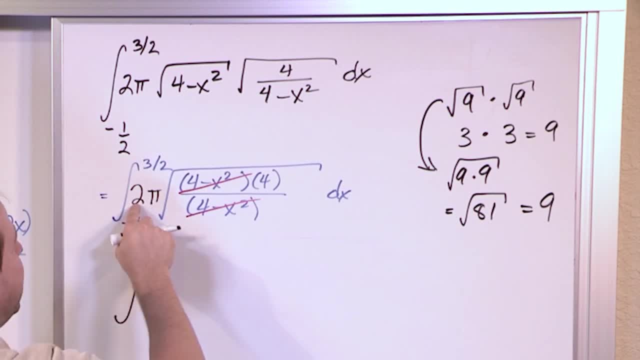 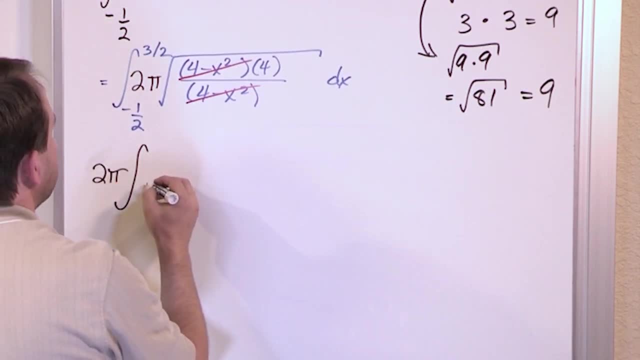 integral of. we have 2 here and we have pi- The square root of this guy. let me just go ahead and rewrite it. You're going to have 2 pi. You're going to have the integral of the square root of 4 dx. That's basically all you're going to be left with. So what? 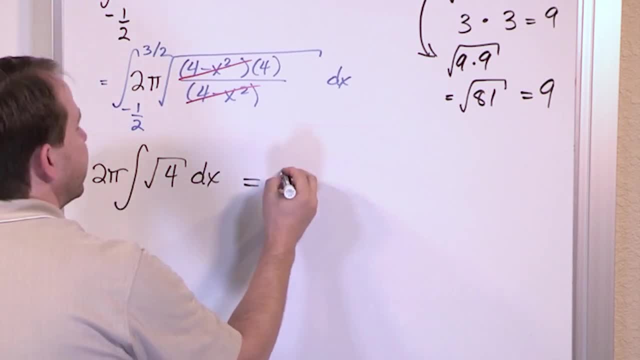 you're going to have this is going to give you a 2.. 2 times 2, when you pull it out, is going to give you 4 pi integral of 1.. Basically, it's going to be left in here, Don't forget. 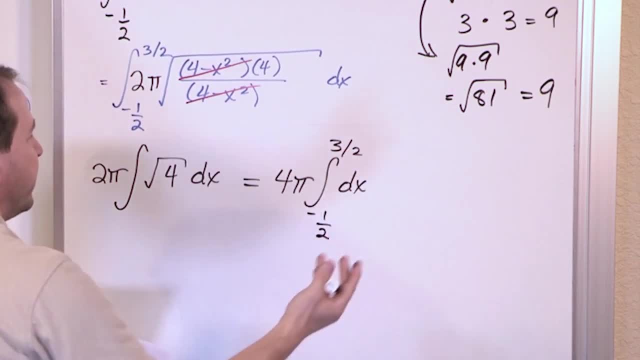 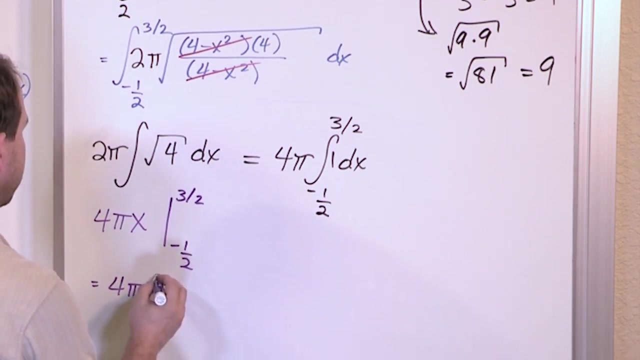 your limits of integration: negative 1 half to 3 half. This integral is incredibly simple. It's like integrating a 1.. So all you have is 4 pi x. That's the integral from negative 1 half up to 3 halves. So you're going to have 4 pi And in here you evaluate the top. 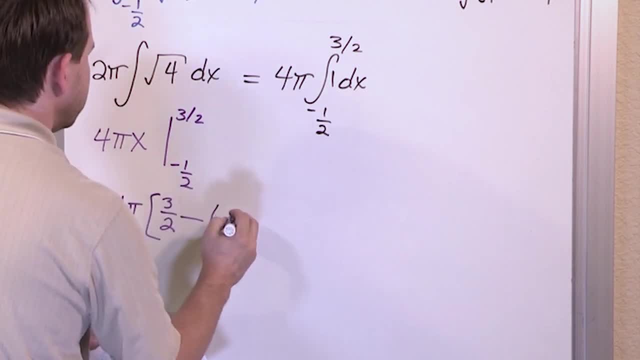 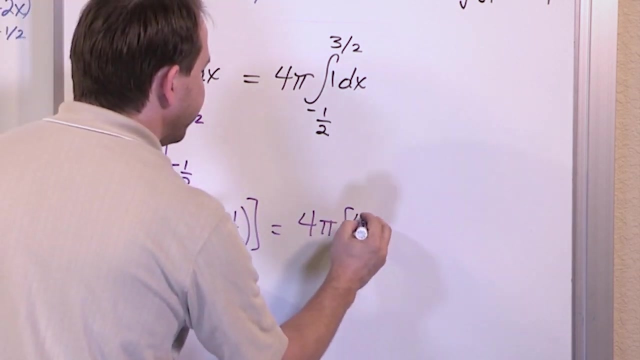 limit, Limit of integration, minus the bottom limit of integration, which is going to be 4 pi. And I have these guys here, So this is going to be a plus. So, since this is a plus, it's going to be 3 plus 1 is 4.. 4 halves, which is going to give you 2. And then you're going. 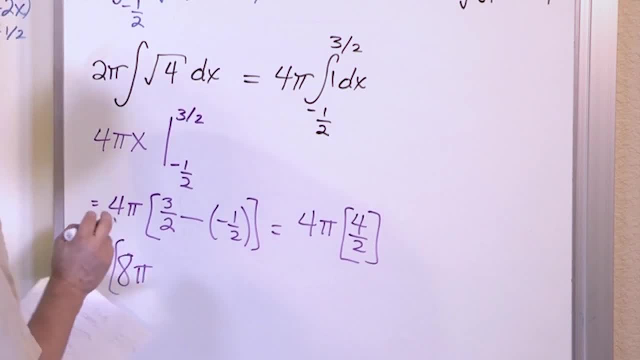 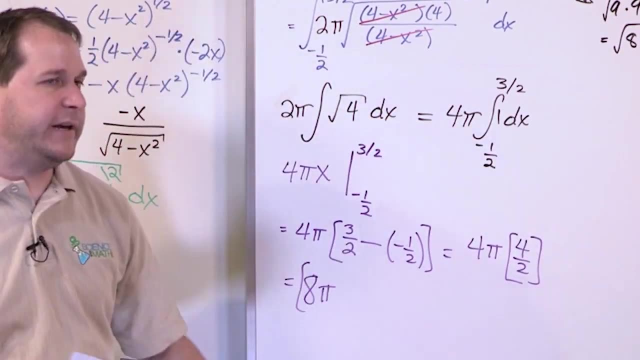 to be multiplying here, So you're going to get 8 pi. 8 pi is the final answer And that's how you handle, You're doing these surface area problems. What would the units be? It would be 8 pi square millimeters or 8 pi square inches, or 8 pi square kilometers, or something like. 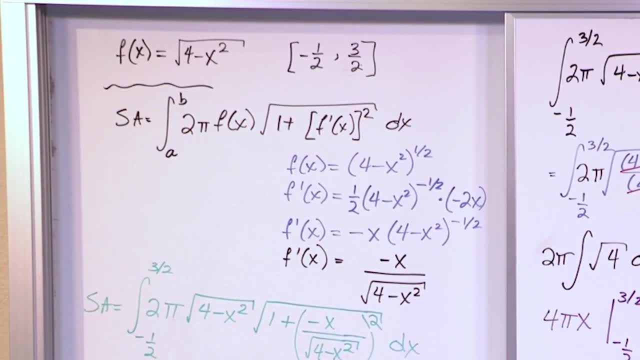 that, depending on exactly what measurements you were using, Like I said, the actual calculus part. you just have to kind of crank through it sometimes and just trust that when you get these crazy looking integrals that they will simplify. You just need to figure out. 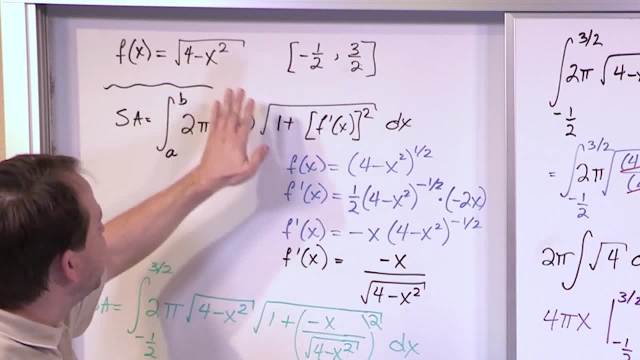 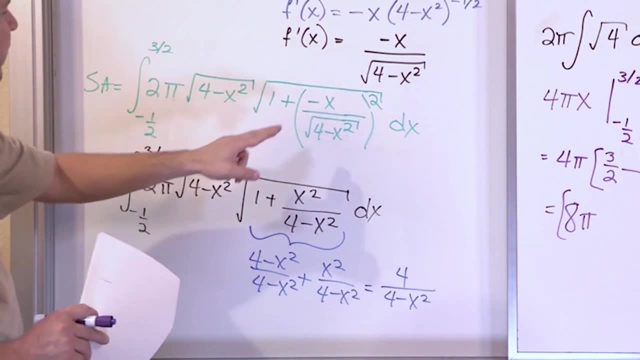 how to do it properly. So you put your function, You take its derivative. Here's what you get: 2 pi f of x Times 1, plus the derivative squared. So then we square that derivative And that basically gets rid of the radical in the bottom And it squares the top. And then we realize we 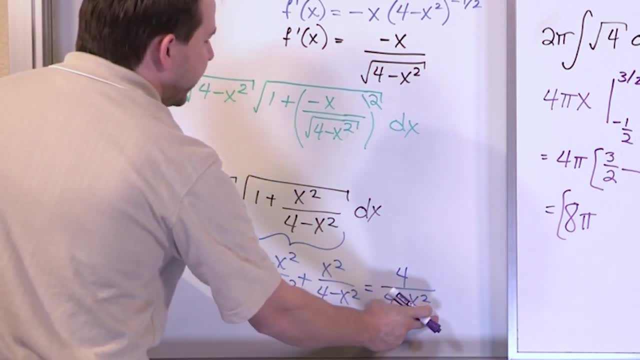 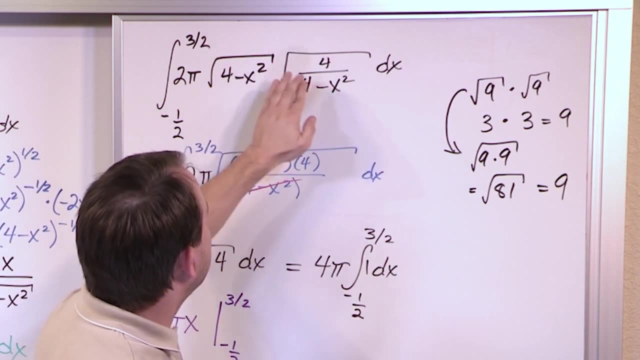 need to combine these together So we get a common denominator. We combine them together And we get this. So this is what is living under the radical here, And then we know that we can combine radicals by multiplying the inside terms together and enclosing the whole. 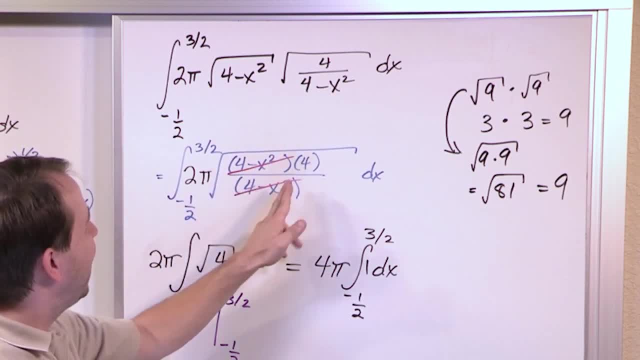 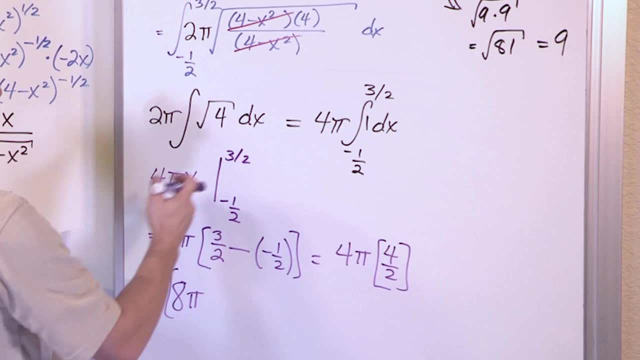 enchilada under a large radical. When we do that, we can cancel half of everything in the problem. That's the beauty of how this thing simplifies. And then, finally, we're just left with the square root of 4. in the inside, We have tons of constants. All the constants come out. 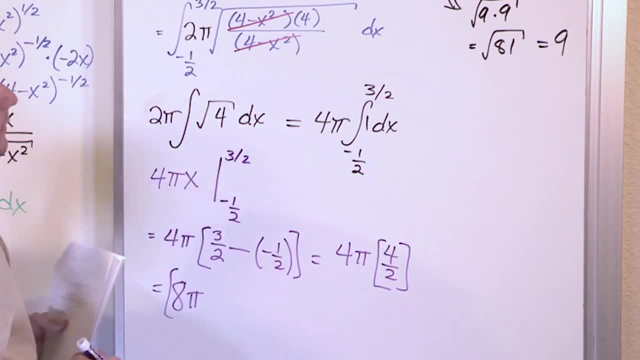 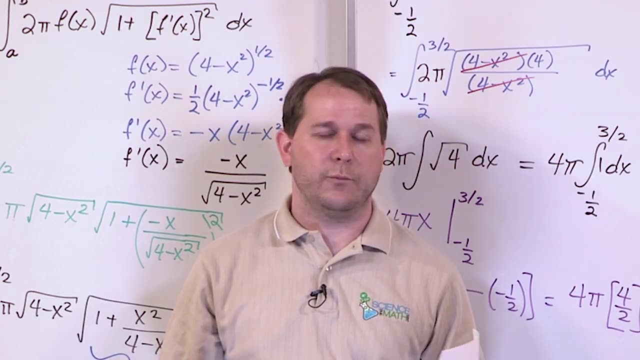 And then we just have a very simple answer to this integral, which we plug in the upper limit and the lower limit and get our final answers. And that's how you calculate surface area. They're all going to work the same way. You're going to be given a function, You're 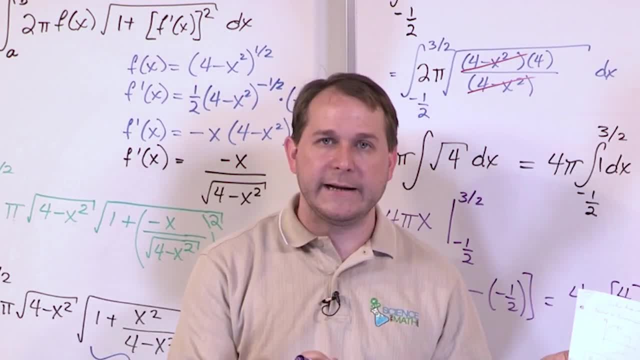 going to take its derivative, You're going to stick it in there, You're going to square it, You're going to combine it And then you're going to just work through a simplification. Sometimes you might have to use substitution, Sometimes it might not, Sometimes it might. 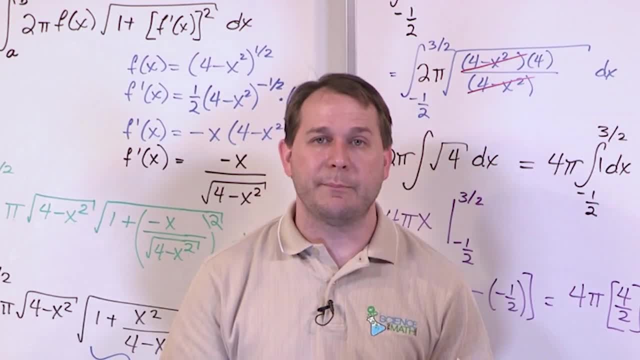 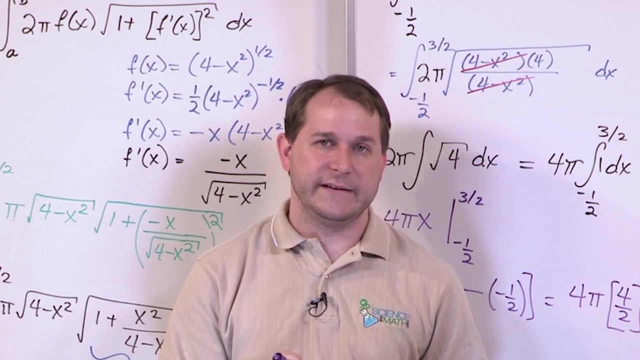 totally fall out like it did in this problem. Sometimes it might become a polynomial, like you might imagine might be able to happen, and so on. So use all the tools at your disposal to simplify these integrals, And one thing you just have to kind of know is that if you're 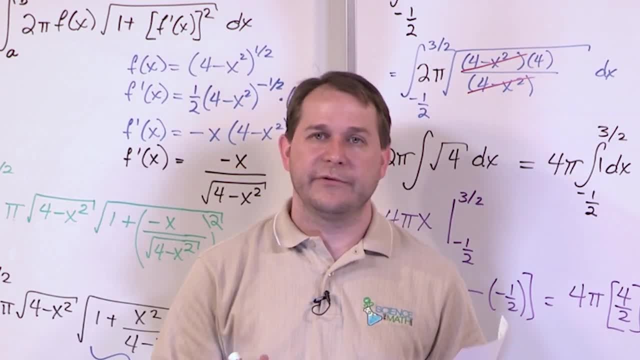 on a test and it doesn't simplify. you just need to roll up your sleeves and find the right way to make it simplified, because it has to. It has to simplify. You're not going to be expected to take integrals of incredibly complicated functions without simplifying. 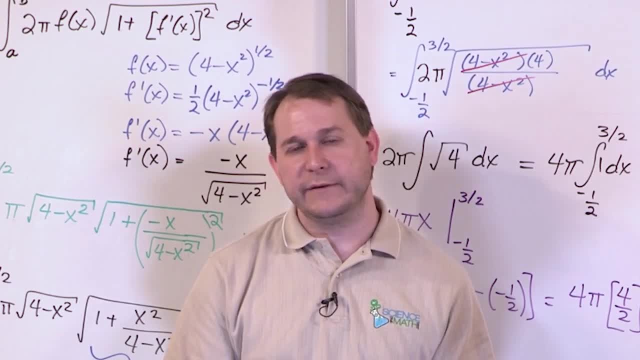 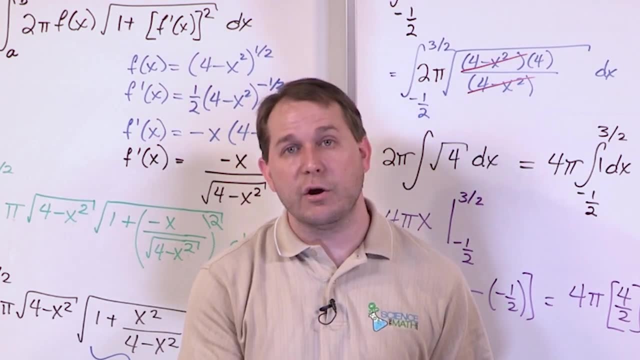 them into something easier to look at. It's just, You're not going to be expected to do that on a timed exam, So make sure that you're seeing some cancellation, You're seeing some reduction, You're seeing some simplification, And then you'll know that you're on the right track. So please understand these problems. 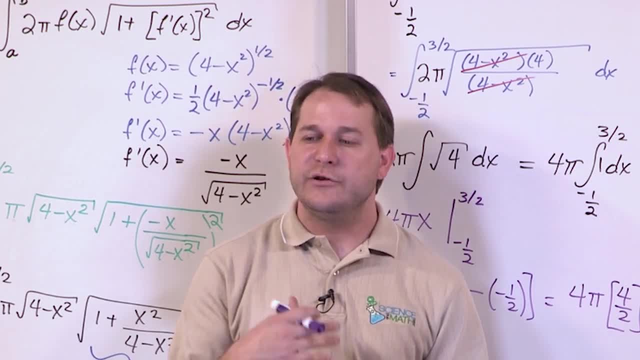 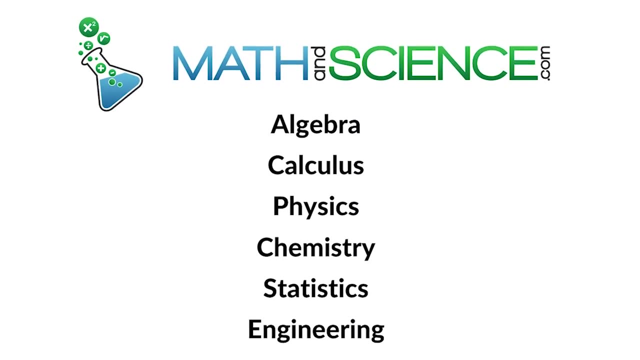 Work them for yourself, Practice them yourself, And then you'll continue to get good at calculating the surface area of an object using integration. Learn anything at mathandsciencecom. 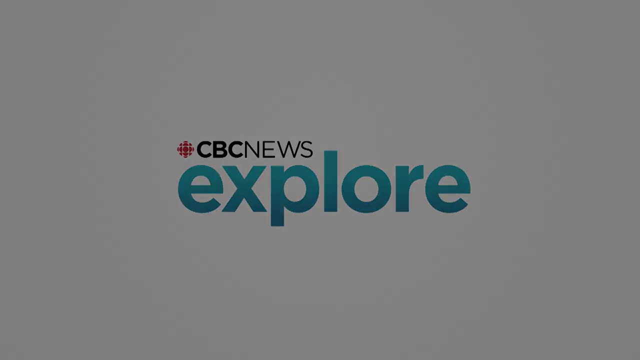 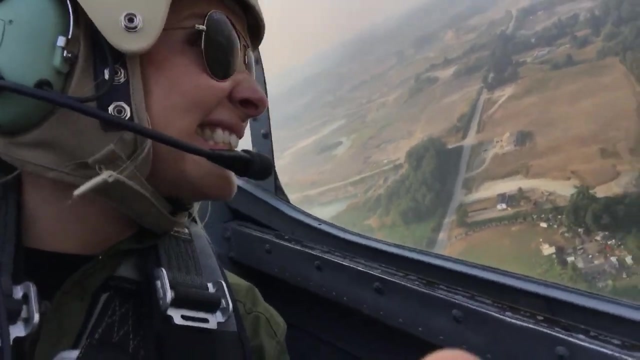 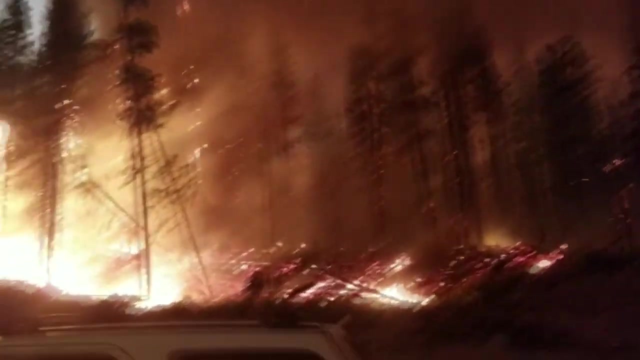 My name is Johanna Wagstaff. I'm a meteorologist and an earth scientist. Every day I see the effects of climate change through my work: A relentless cycle of extreme weather, terrifying storms, deadly heat, domes, wildfires, droughts. But I remain in awe of the natural world, and how. 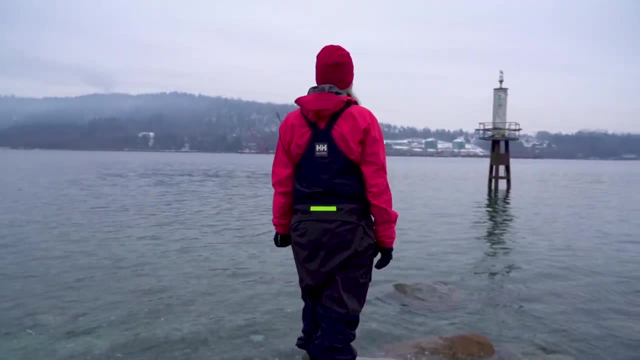 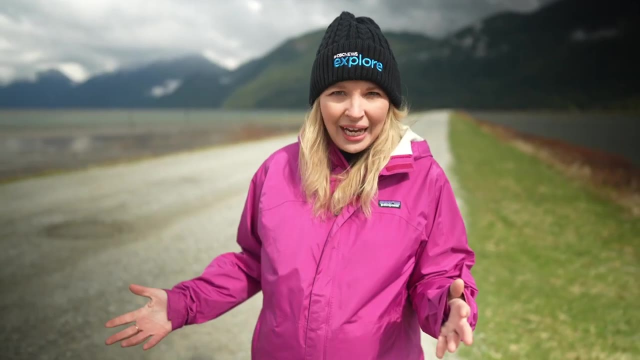 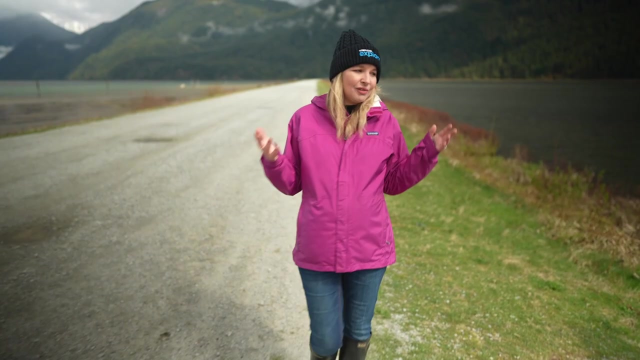 it finds ways to adapt, And that's what we explore on Planet Wonder. Polar vortex, atmospheric river heat dome. We know these weather phenomena connected to the jet stream are changing, So that got me wondering what's going on way up there that makes weather.